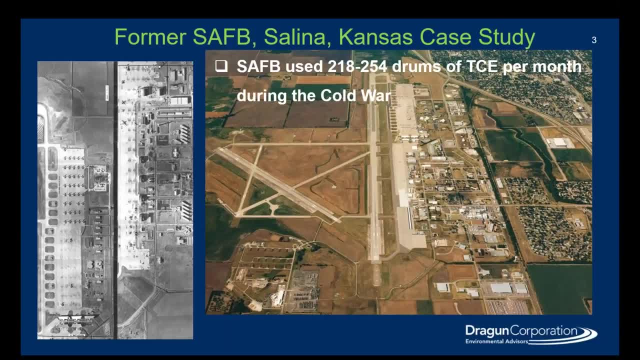 So at this line Air Force Base is 218 to 254 drums of TCE per month. This was a lot more than other bases, much more than other bases. So what Well? the groundwater is moving to the city water supply and people live and work above where the groundwater is impacted by TCE. 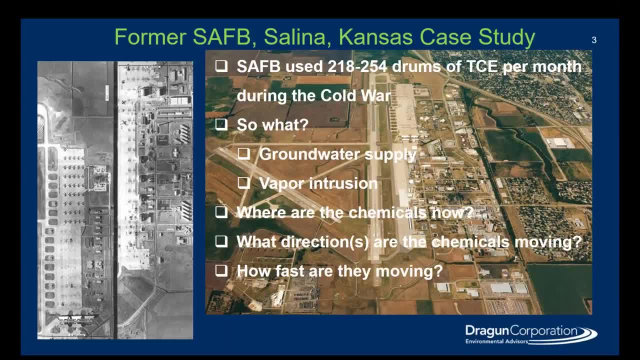 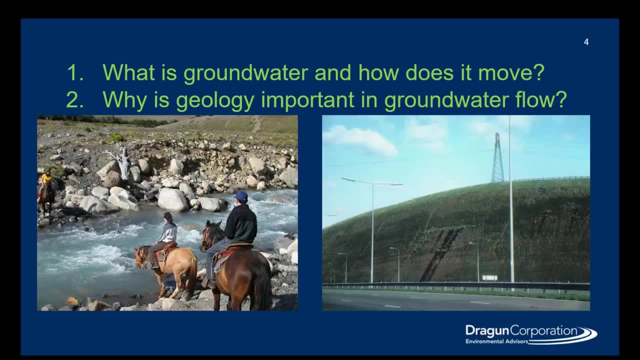 So where are the chemicals now? What directions are the chemicals moving, How fast are they moving And how do we clean it up? So we're going to look today at groundwater and how it moves and why geology is important In groundwater flow. we're going to talk about geology first, focusing on the very basics for both. 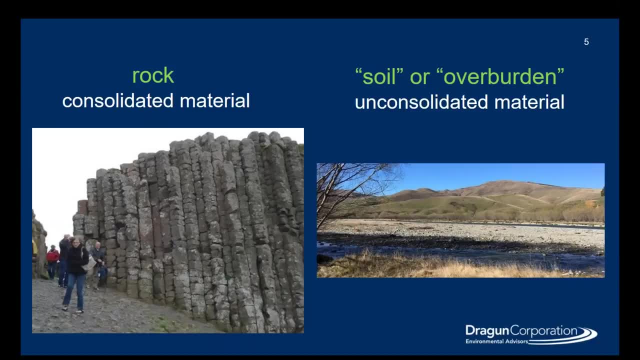 So we broadly can classify geologic materials into rock and soil, or sometimes we call soil overburden. Rock is consolidated material. That means that it will hold up and not fall down. So that means that it will hold up and not fall down. 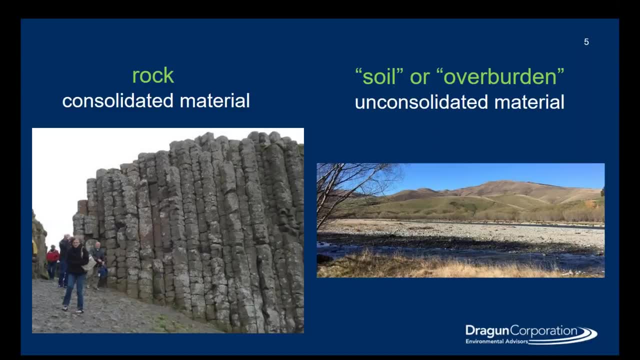 So that means that it will hold up and not fall down. So that means that it will hold up and not fall apart if you put a piece in your hand, for example, Whereas soil is unconsolidated, meaning it will fall apart if it's dry in your 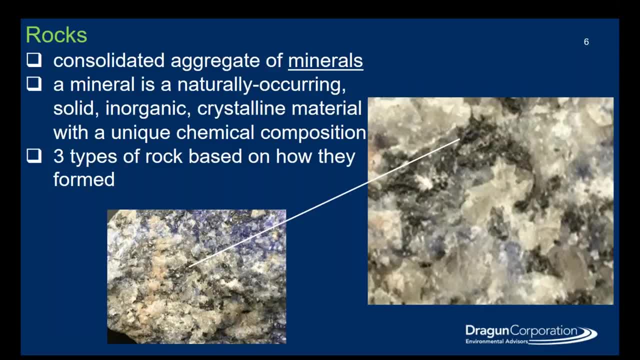 hand. So rocks are consolidated aggregate of minerals, and a mineral is a naturally occurring solid, inorganic crystalline material with unique chemical composition, And in this slide we can see the- I've got a close up over on the right. This is a mineral, a dark mineral that 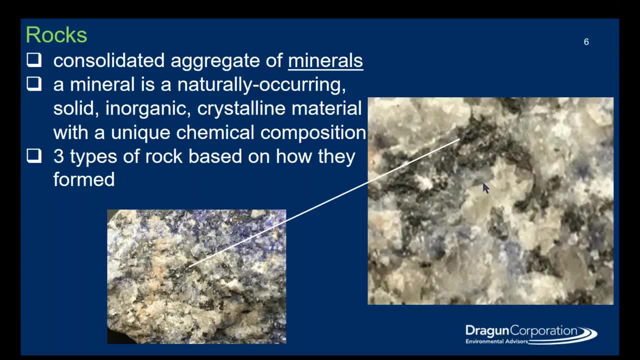 you're seeing, And you can see the interrelationship of the various crystalline minerals- that there's no space between the minerals. This is common in many rocks and it affects whether groundwater can be present and moving. So there are three types that we're going to talk about. 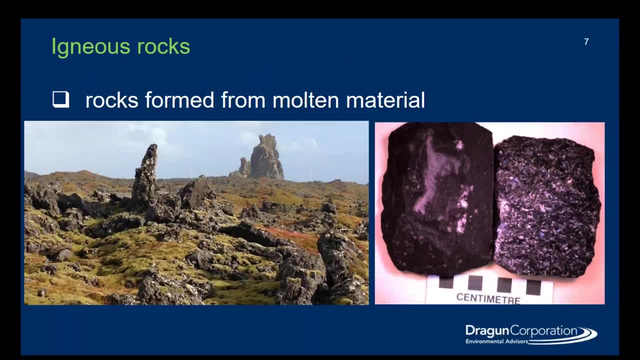 The common rocks based on how they are formed. The first one is the most recognizable of the igneous rocks. what we're seeing here. Igneous rocks are formed from molten material. The picture on the left is a landscape from Iceland. The rock on the left side of the photo on the right. 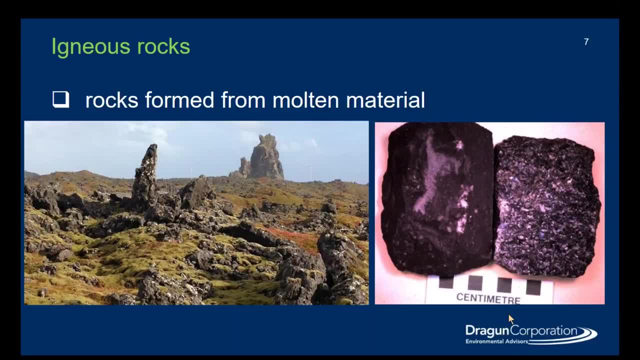 the dark rock with. you can't see individual grains in. it is an igneous rock from a volcano. The rock on the right on the right photo you see individual grains of minerals. This is formed deep in the earth. It's also an igneous rock. The common elements from a groundwater perspective. 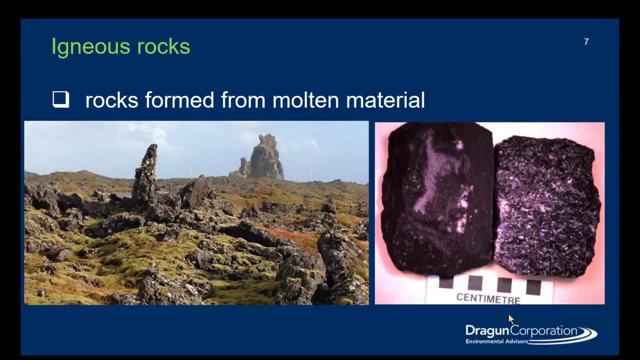 is, the grains are interlocking. There's virtually no space for groundwater to be and groundwater to move, And that's what we're going to talk about in the next slide. And then we're going to talk about the other types of rocks that may be present, And that's why we're going to discuss a little bit. 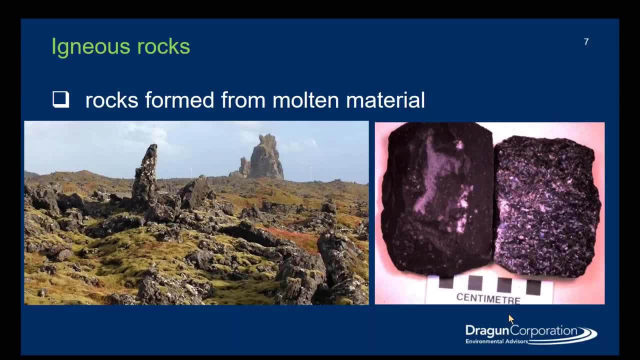 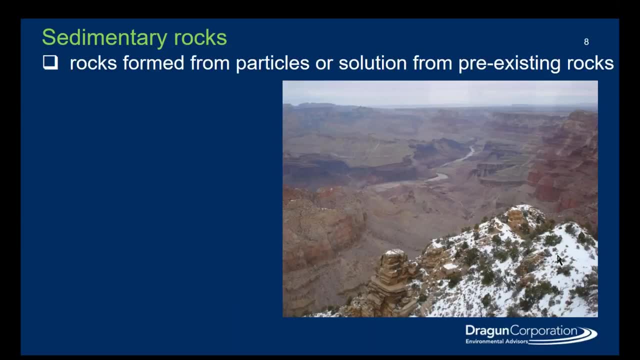 about this more in the future, But we should point out, in some volcanic landscapes like Iceland or Hawaii, there's larger-scale volcanic features that can support groundwater flow. The next type of rock body method of formation is sedimentary rock. Sedimentary rocks are formed from particles. 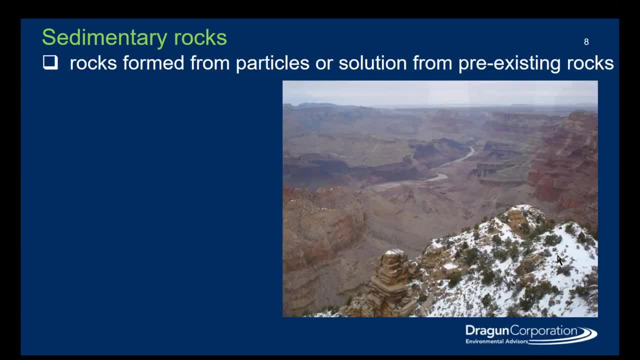 or solutions from pre-existing rocks. The picture on the right is from the Grand Canyon And this depicts typical things we see in sedimentary rocks. They're laid down in layers. They're typically light in color. Sedimentary rocks can form either from particles, where there's space in between. 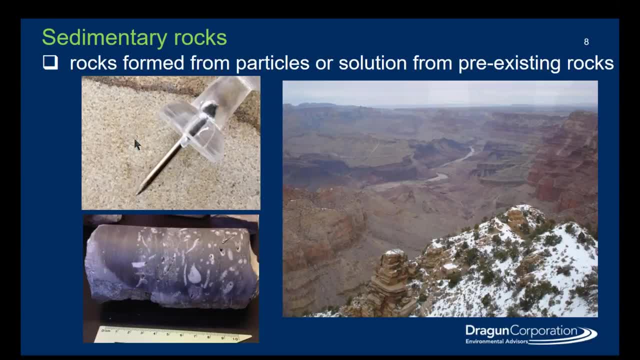 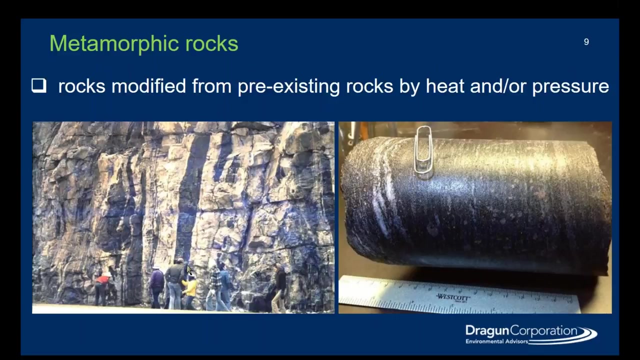 And on the left side we see sandstone made up of quartz particles coming from pre-existing rocks, And on the bottom we see limestone. You can see shell pieces that come from pre-existing materials. The third type of rock, by the way it's formed, is called metamorphic rock. 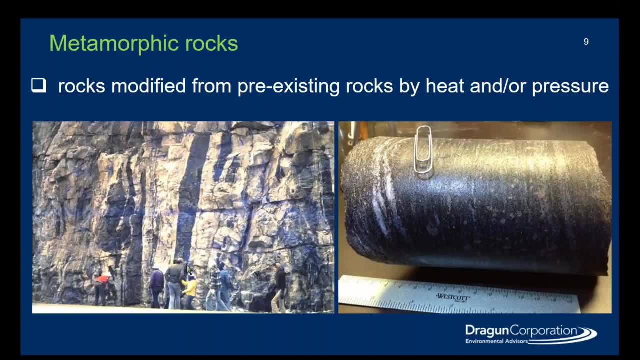 These are rocks that are formed from pre-existing rocks and changed or metamorphosed due to heat and or pressure. They're generally formed deep within the earth And, as a result, we see things like rocks being pulled apart by the stresses in the earth as they're heated up. 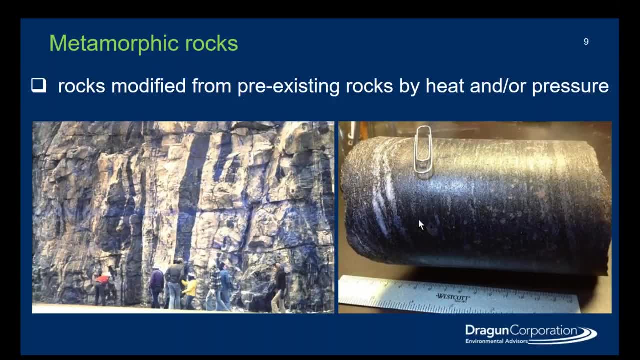 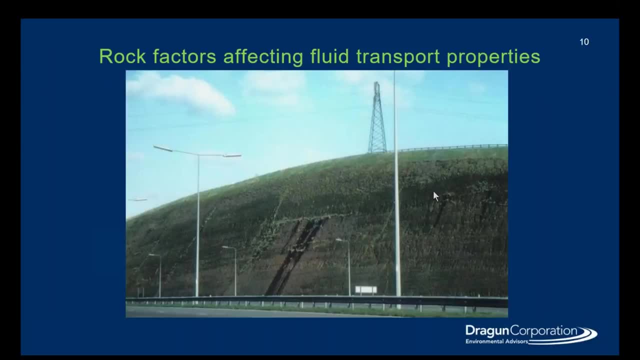 And on the right we see that there's very little space. The grains are interlocking and that precludes a lot of groundwater flow. So what are some of the factors that affect fluid transport in rocks? And, as we mentioned, the grains are interlocking generally. 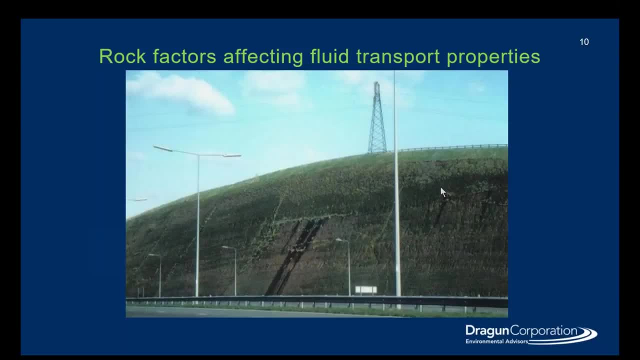 and, as a result, they're not capable of transmitting groundwater from many types of rocks. But secondary features can form, like we see in this road cut where there is a fracture or a break in the rock through which water is seeping the dark areas that you see. 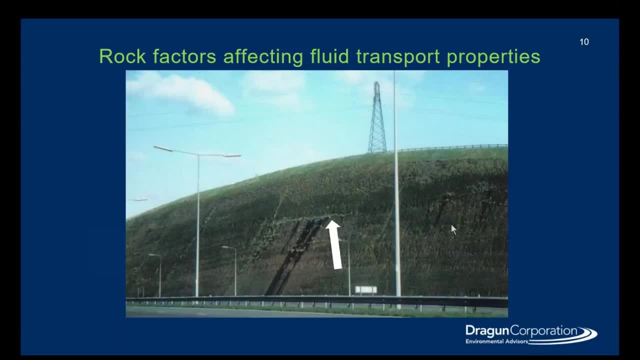 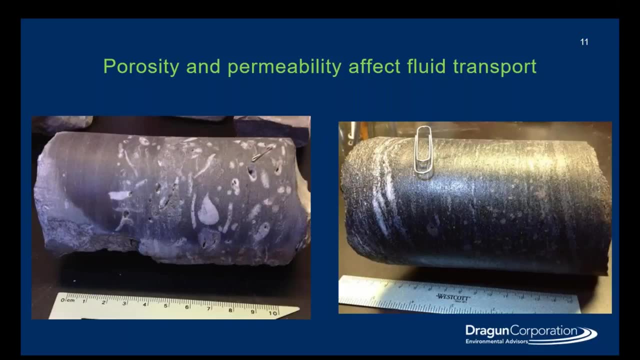 And that's one of the ways in which rocks can transmit water. So the two main factors that control fluid transported groundwater in rocks is porosity and permeability. Porosity is the ability to store water, meaning void spaces, like we can see void spaces in this rock on the left. 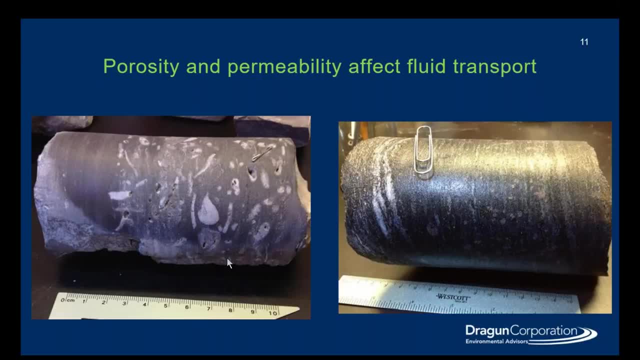 And permeability refers to the ability to move water, And that relates to whether the pore spaces are interconnected or not. Another term for permeability that you may see is hydraulic conductivity. In general, rocks have little to no porosity and very low permeability, as they're originally formed. 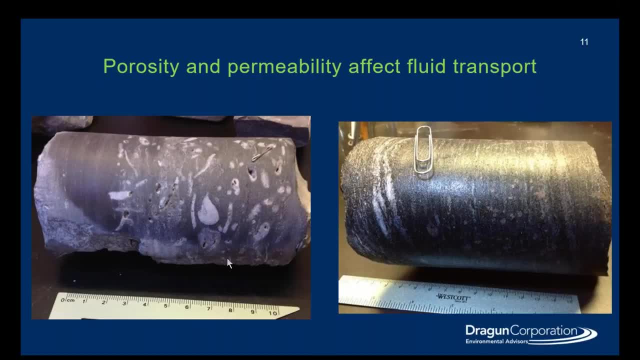 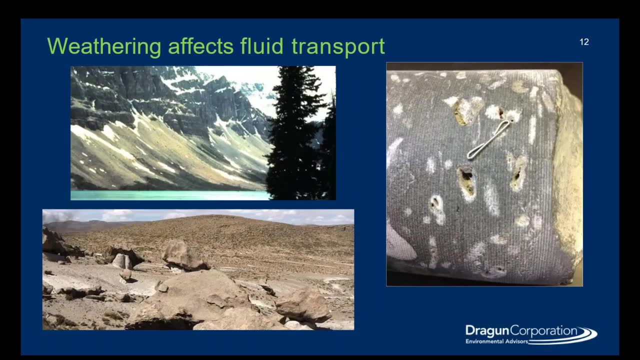 But if they are affected by post formation and conditions, they may be able to transmit water, And here we see some examples of processes that can change the ability for rock to transmit water. This is called a talus slope here. This is rock has been falling off this face. 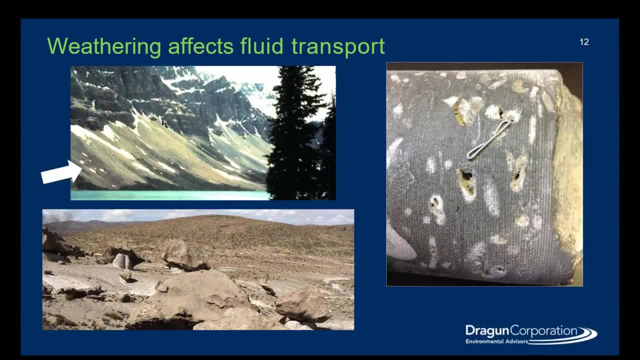 of limestone mountains in the Rocky Mountain area of Canada. On the lower one we see rocks that are affected by weathering, by really abrasion, in the Peru high desert, And on the right we see a core of limestone that has been dissolved in certain areas. 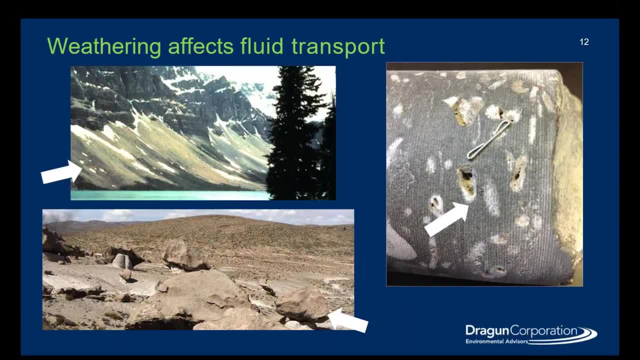 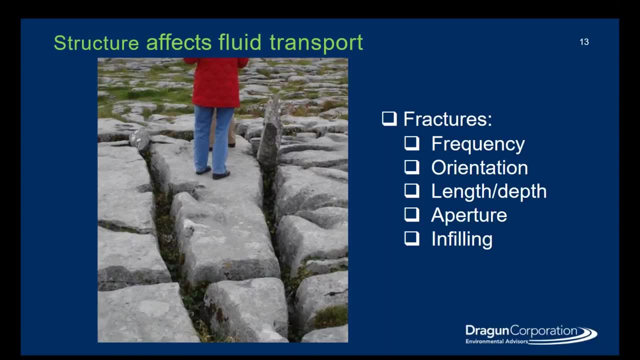 And that has affected its ability to transmit water. What that means is that it's a very important factor in bigger volume And the structure also affects fluid transport in rocks and it can be a very major factor. Fractures are simply breaks in rock. 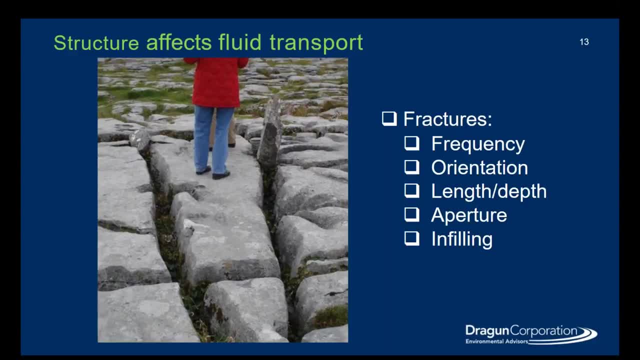 that have occurred due to stresses or cooling, But there are a number of characteristics of the fractures which will control the ability to transmit fluids. How clean is the air? frequent are they? how many fractures? what's the orientation of the rock? is that will affect the 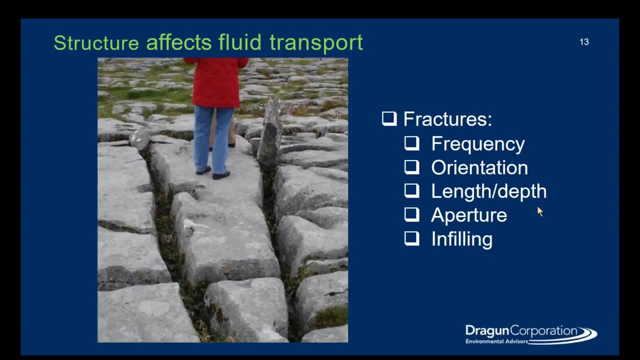 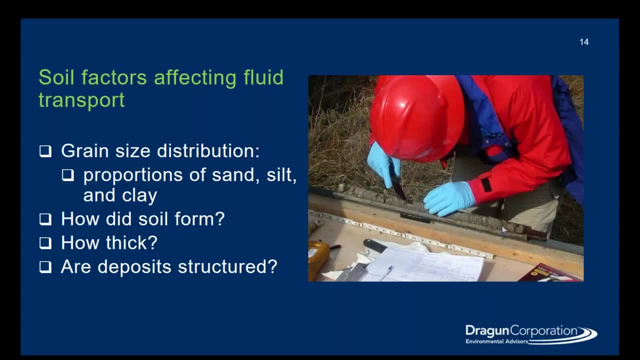 way groundwater may move? what's the length and depth of the fractures? what's the width of the fractures, the aperture, and are the fractures in film? look. now we're going to look at some factors that affect fluid transport and soils. soil is the main property that controls water. 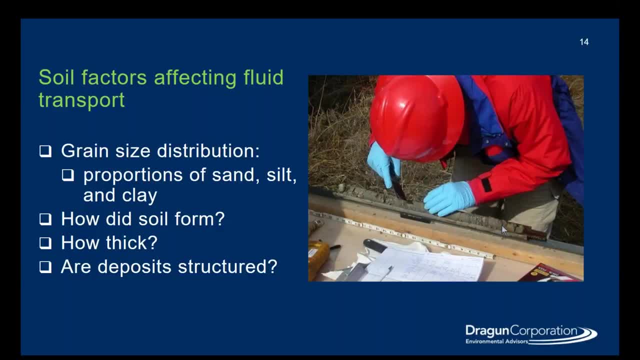 movement in most soils is the grain size distribution, meaning the proportion of sand, silt and clay sized particles. the more fine particles like clay you have, the less likely the soil can transmit water. and then there are some other uh factors. how did the soil form um? how thick are the deposits? you know the deposit structure and that means do they have? 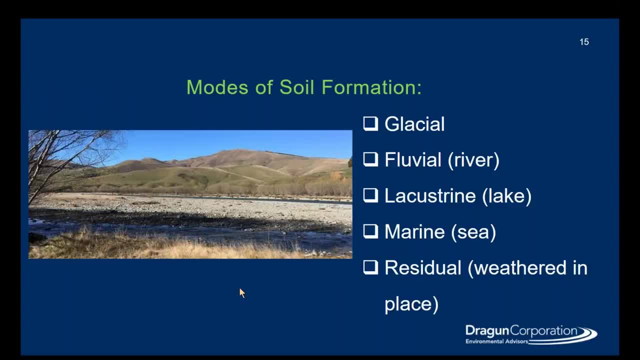 uh, features that occurred after the soils were formed. so how were? how can soil be formed? well, here are some of the major methods: from glaciers, fluvial means- they're river deposits that, like we said in this photo, uh lacustrine uh are lake deposits, marine or sea deposits, and residual soils are. 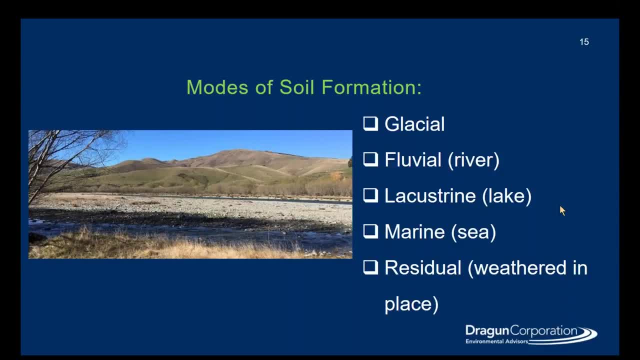 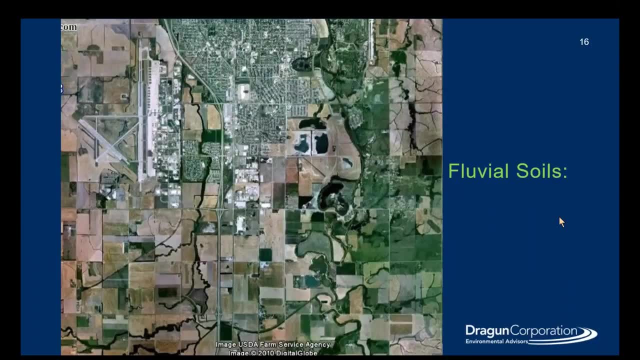 those that are weathered in place, so they're in, they're not moved at all. where these other ones are moved from, where the rock originally was fluvial soils are, are very can be very complicated, and this is a site that we've been working on when i mentioned in kansas and 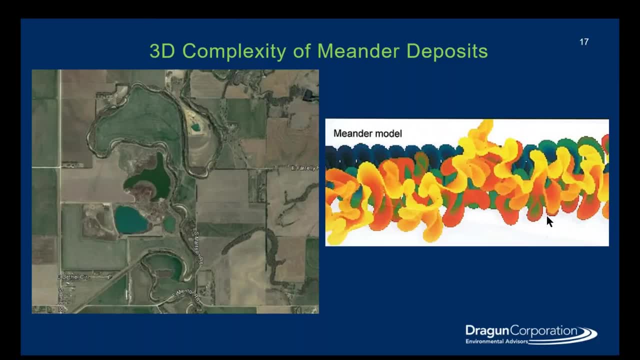 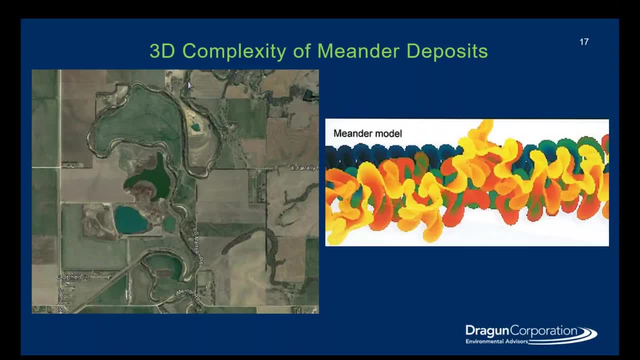 us characteristics and in different spots. this is an area where this is kind of the inside of a meander loop and that's where sand would be deposited, and the blue arrow it's the outside of a meander loop where materials would be eroded. this, the white arrow, indicates a meander where that could be cut off in a storm. 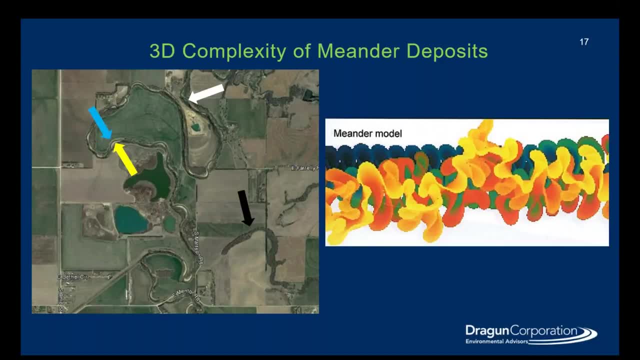 and basically isolate that meander loop, and the black arrow shows an old meander loop that has been cut off and the reason that's important is that the water that is gonna be the shell and the material that is going to bring in could doesn't move very readily in these cut-off meander loops. 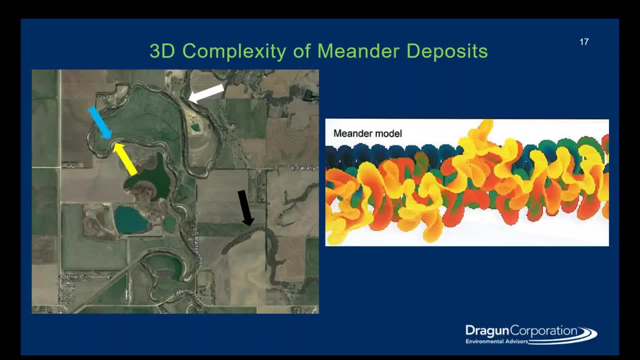 And you would get clayey types deposits there. So because of these different parts of meander loops in two dimensions, you get various types of material being deposited in various areas, But the meander model on the right- and I apologize because I can't find the source- 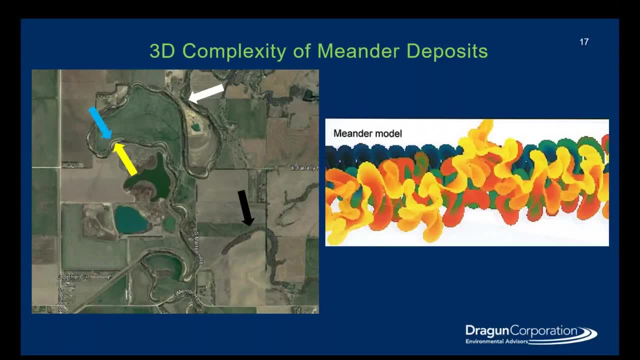 of where I got this picture is showing the meanders in three dimensions. The yellowish colors are the most recent ones- on top We're looking from above- and the dark colored ones are the older ones, So they formed at an earlier time. 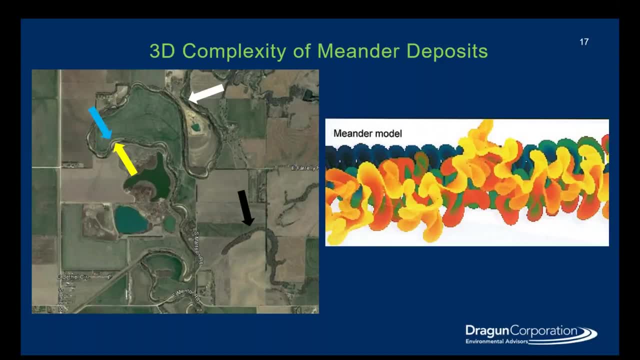 and they've been covered by later deposits. Well, the thing here is that you could be looking in the recent deposits at a place where sand is deposited, but below that it will be an area that there might not be sand. So in three dimensions they're extremely complex. 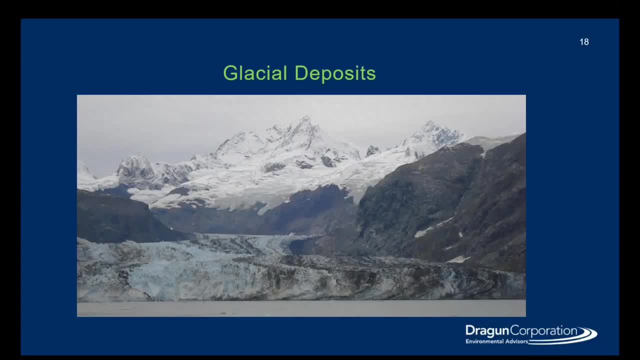 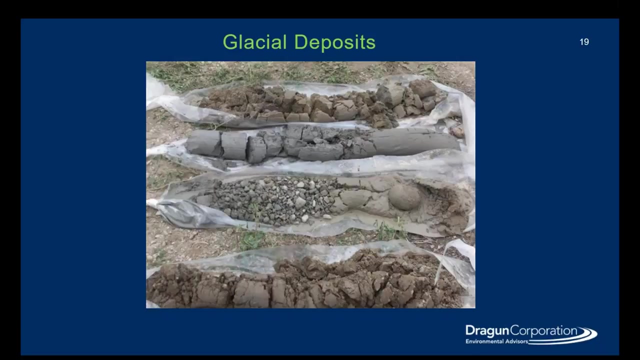 Some discussion about brownfield monies. Glacial deposits are deposits that are laid down either by alpine glaciers, like we see here, or by continental glaciers that now exist in the Northern Arctic and in the Antarctic, And these deposits can be either directly laid down. 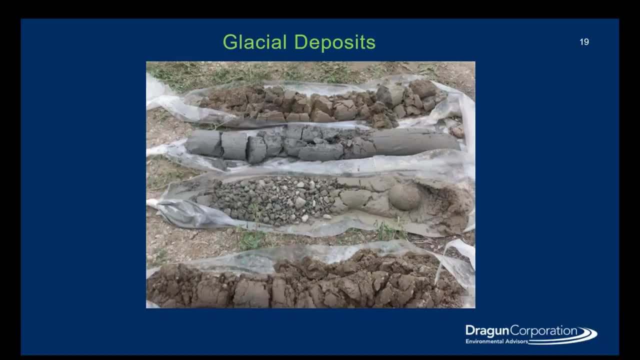 by the glacier or laid down by water associated with the glacier, and they can be very complex. This is a core from Michigan where we're looking at glacial deposits And you can see the yellow arrow is pointing to the bottom. It's pointing to an area of sand. 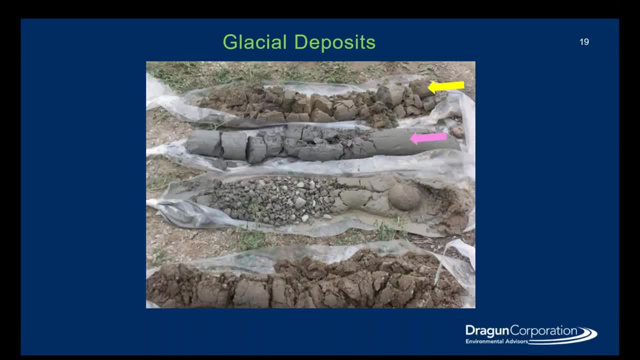 And the arrow below it is pointing to an area of clay. So this is all in a vertical profile And then the white is showing gravel. So you can have a lot of complexity in geologic materials. And the white- the gravel- would transmit water fairly well. 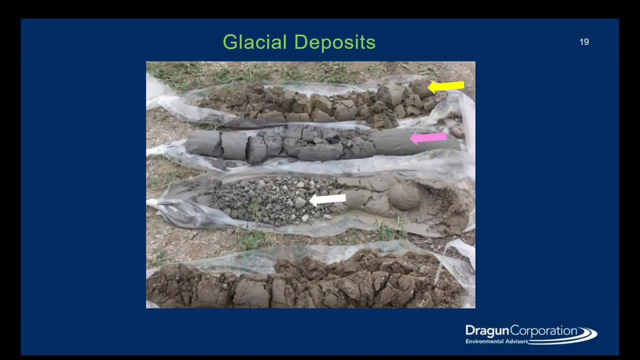 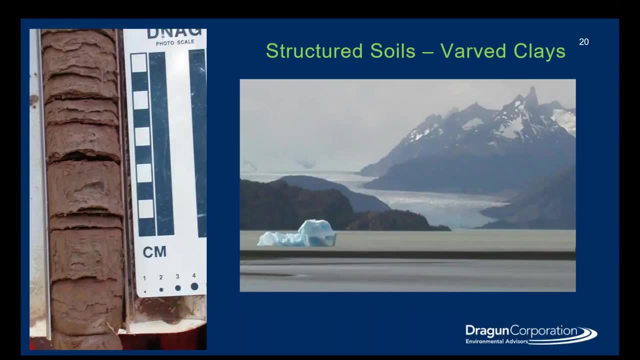 But the intervening or would not, because it's mostly clay. Another thing you can get from glacial deposits are barb clays, And this is a barb clay that we see on the left, And barbs are kind of rhythmic deposits. 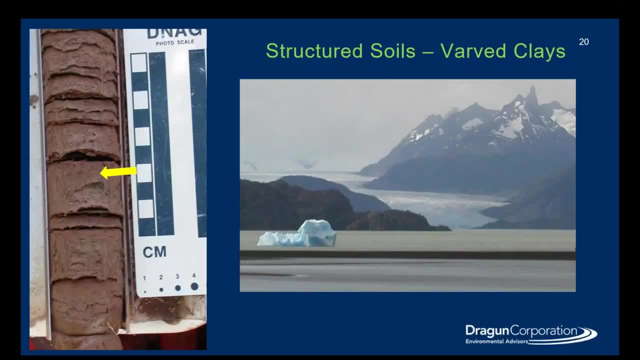 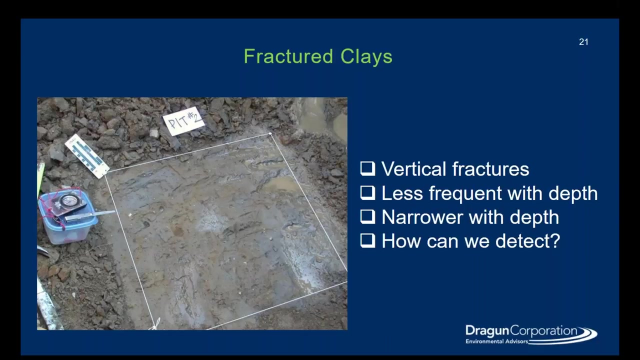 that you get in glacial lakes, with the finer materials deposited during cold episodes and the coarser materials being deposited during high flow episodes. But what you see in a vertical direction is a lot of variability. You also have fractures in soils. These are fractured clays in Ohio. 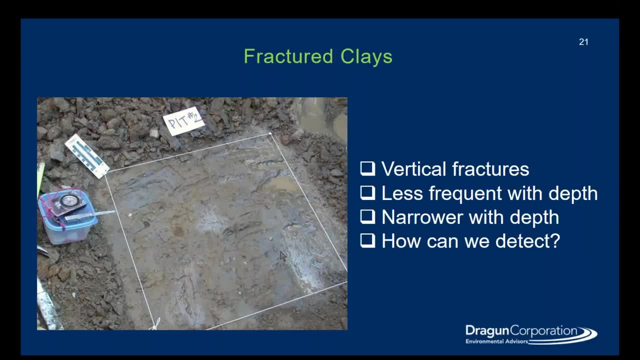 And you can see on this slide that most of the soil is clay and doesn't transmit water, But we can see these wet areas where the clay is fractured, And these fractures are vertical so they're difficult to locate or identify when you're working in a fractured clay area. 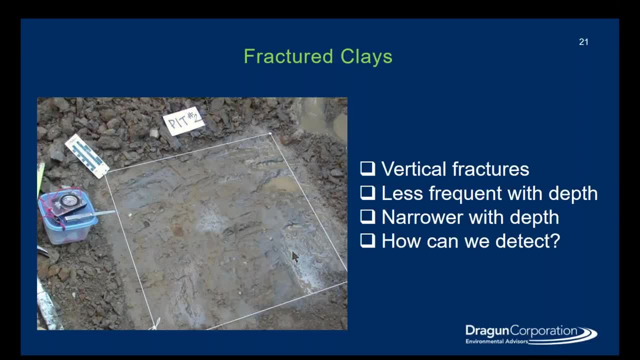 because they become less frequent with depth. they become narrower. with depth the aperture closes up and they're vertical. So if we're drilling vertically, it makes a problem. So how do you think that you could identify these if you're in an area where these are common? 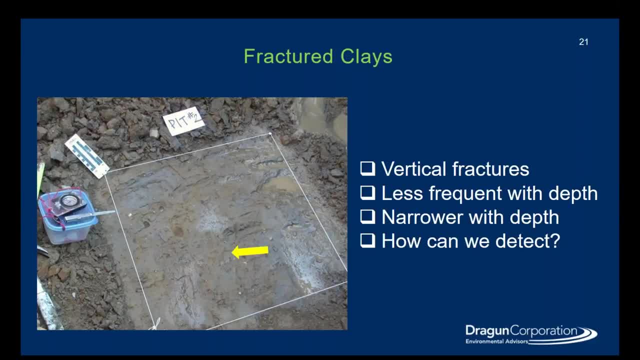 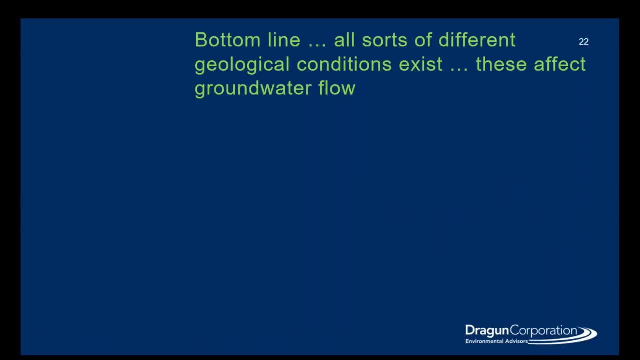 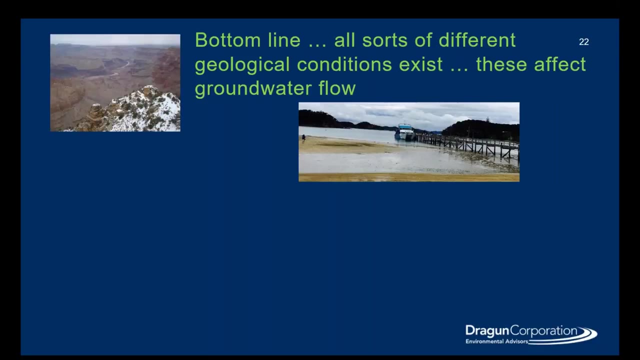 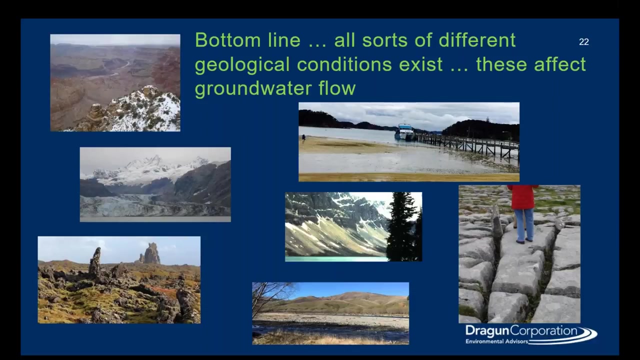 And it makes the ability to transmit water significantly different. So there's the. So the bottom line is there's all sorts of different geological conditions and these affect groundwater flow. So you need to understand the basics of the geology in order to know whether you're going to have a lot of groundwater flow or not. 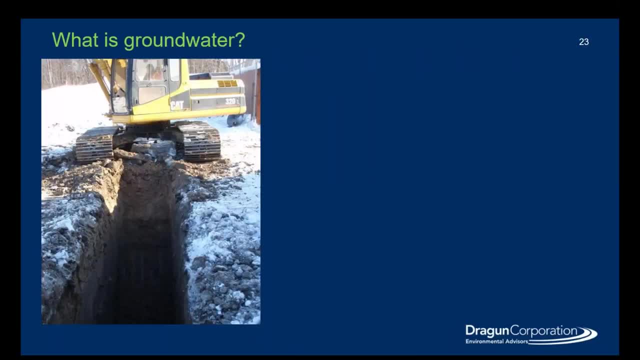 and what the controls on the groundwater flow are. So we're going to move into the groundwater portion of this webinar, And the question is: what is groundwater? Well, groundwater is all water below the Earth's surface. So, no matter where you are, if you dig deep enough, you're going to run into groundwater. 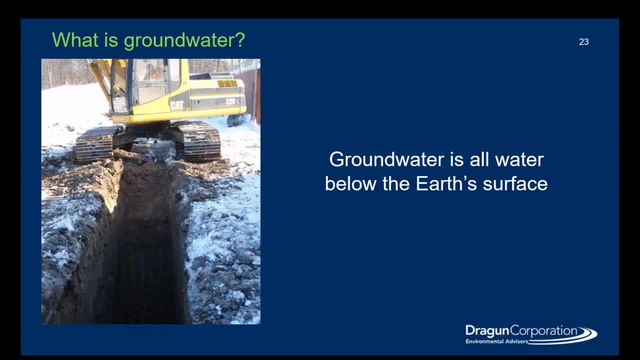 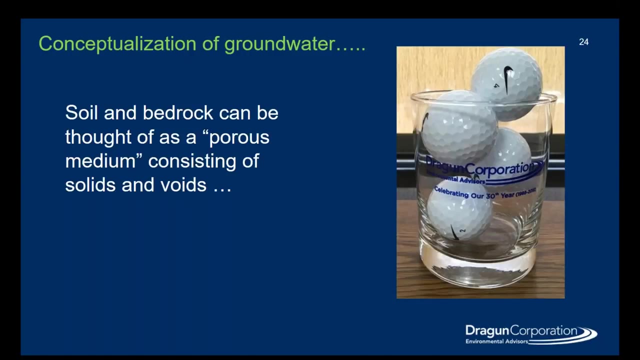 unless you're in very, very, very dry areas or kind of unfractured rock. But you'll find groundwater. Sometimes it can be very close to surface, Sometimes it can be hundreds of feet below the surface. So this is a conceptualization of how groundwater looks. 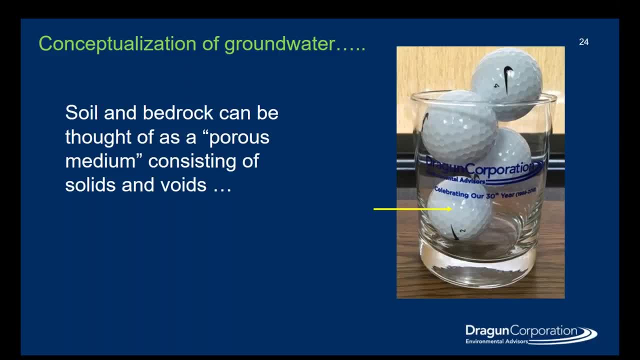 Soil and bedrock can be thought of as a porous medium consisting of solids, which are the golfballs in the glass and void space, which are the spaces between the strings and the water. andㅋ conversations rooftop again- particles. so that would be kind of the matrix in which the groundwater would 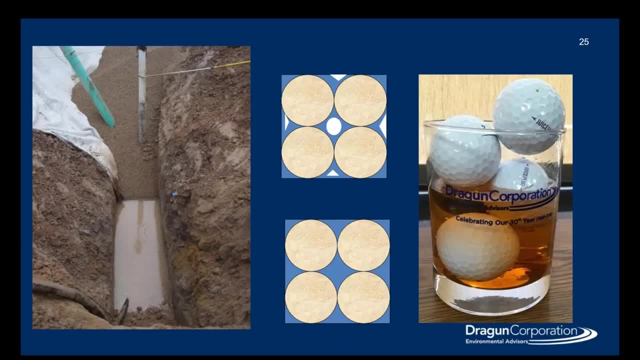 exist and then you just add water and you've got groundwater in a porous medium. this is kind of what you see on the right with this is actually T, if you were wondering, filling up the pore space, but not the solid space. so the water table is a term we use- is the level to which the water fills the pore space in. 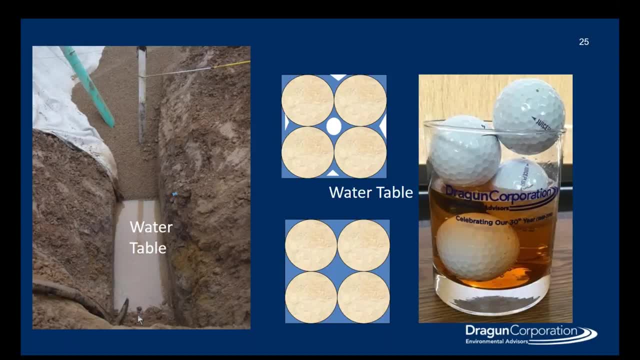 general and we can see that in a hole that we've done here. so the walk that's the top of the what we call the saturated zone. so if we look on this little cartoon with the circles representing the solids, all the void space between the solids and the pores, and the pores and the pores and the. 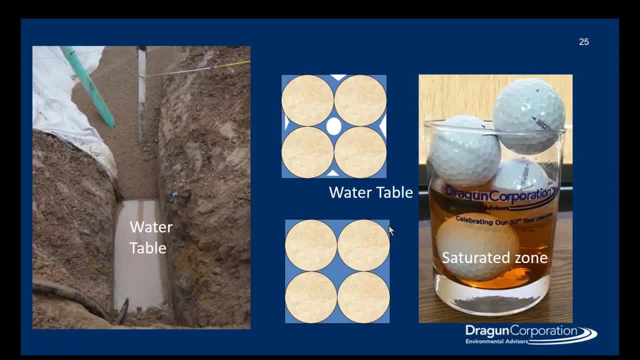 solids is filled with water in the saturated zone but above the water table. if you were to look at that and what's going on, the unsaturated zone and parts of the pore space between the solids is not filled with water and that's generally what we see above and below the water table. so we're looking at this. 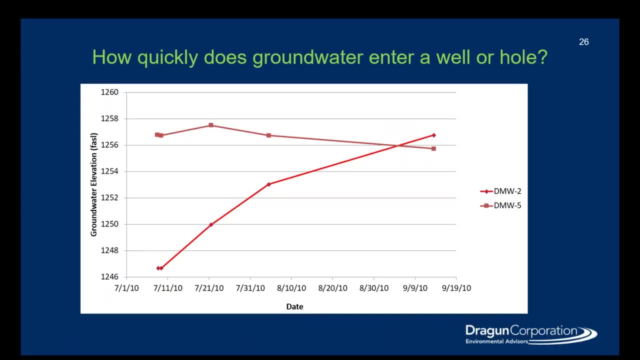 hole. one of the questions you may have is: how quickly does water enter a hole? and this is a graph from some wells that we were looking at at a site where we've we've drilled a hole, and these graphs are showing how the water level rose with with time, and you can see some. 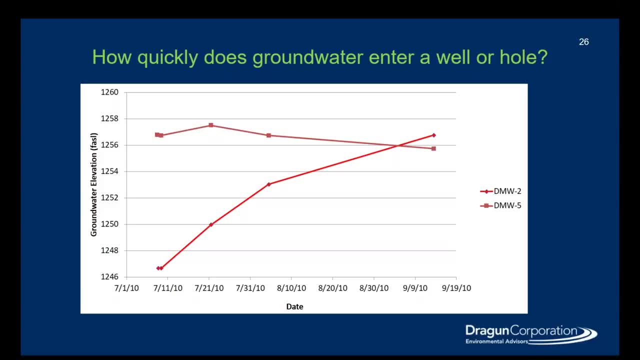 of these took two months to rise to a level. others were right there and and the rate at which the water fills the hole depends on the geology. if you've got things like clayey soils- very fine grain, the water- it takes a long time to enter the hole or the well, and if you've got sand, it can come up right away. 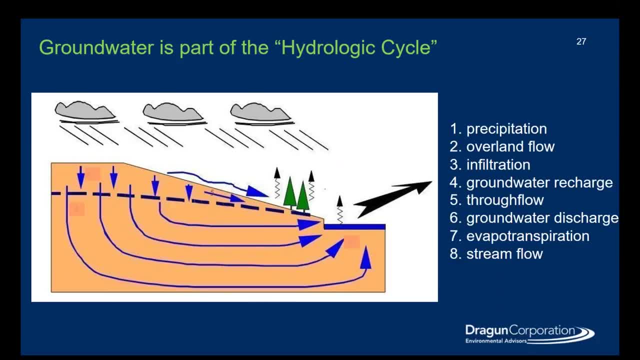 so groundwater is part of a continuum that we call the hydrologic cycle, which is the cycle of of water coming from precipitation. it falls on the ground. some of it runs off as overland flow, other infiltrates into the ground. Four is groundwater recharge. 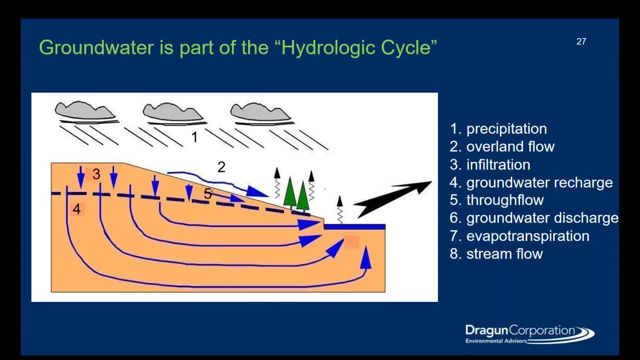 meaning the water actually reaches the water table. Five is through flow, that's, water moving above the water table in the unsaturated zone. Six is groundwater discharge, where the water comes out into the surface water body. and seven is evapotranspiration. 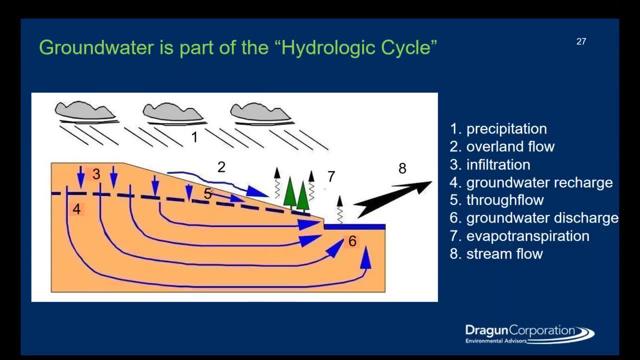 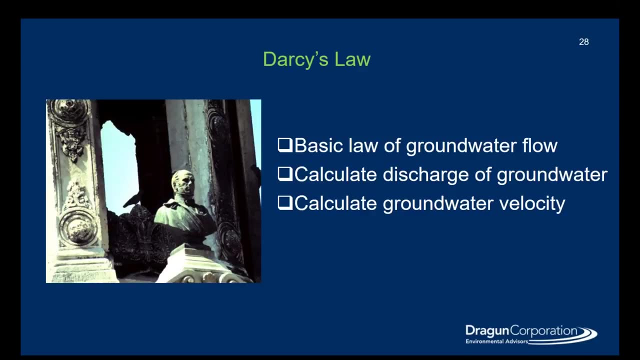 That means the water given off by plants, and eight is stream flow or lakes. So groundwater is just part of the movement of water between number four and number six. The way that we determine groundwater movement, we use a basic law called Darcy's law. 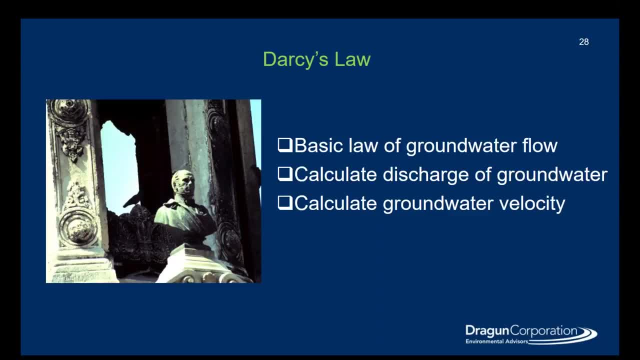 Darcy was a French civil engineer in the 1800s who worked on water supply in the Dijon, France. He came up with this equation that allowed us to either calculate the discharge of groundwater, and we've changed that to also allow us. 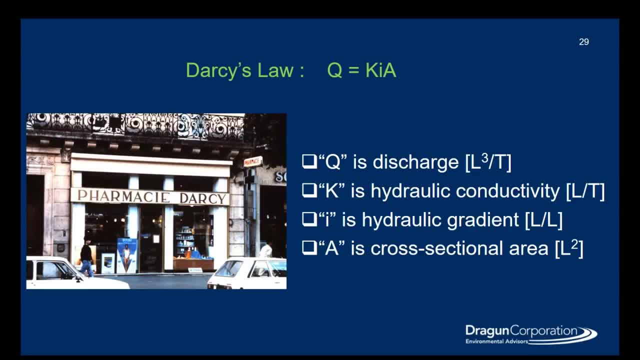 to calculate groundwater velocity. So this is the basic form of Darcy's law Q, the discharge is equal to the hydraulic conductivity or permeability times the hydraulic gradient, small I times cross-sectional area, And we'll take a look at these later on. 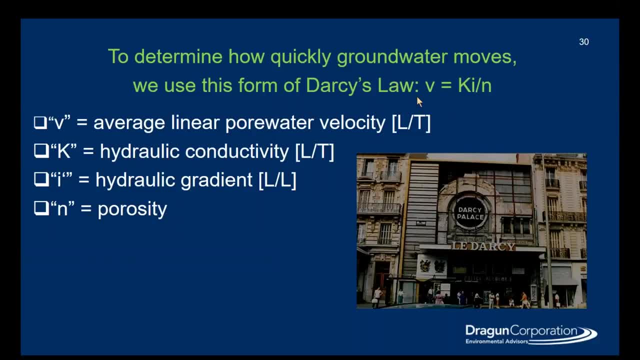 But to determine how quickly groundwater moves we use this form of Darcy's law: V is the average linear or velocity, or the average groundwater velocity, and is the hydraulic conductivity, I is the hydraulic gradient, N is the porosity. So we use this to figure out how quickly groundwater moves. 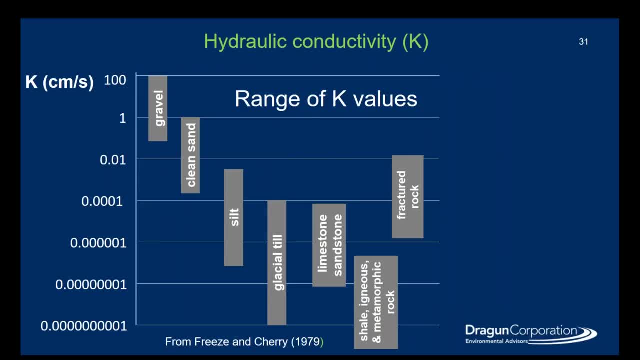 And from that we can figure out how quickly chemicals move in the subsurface. So hydraulic conductivity has got a huge range- 13 orders of magnitude- from gravel, which is very permeable, down to different types of rock that virtually don't transmit water at all. 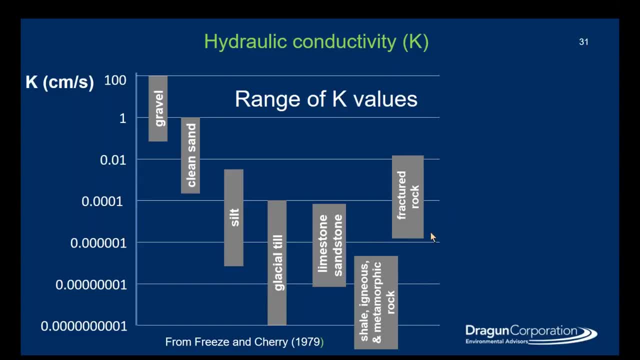 And you can see the rock that's fractured would be more permeable, and so on. The huge variations in hydraulic conductivity depend on the geology, And that's why it's so important to characterize the geology correctly, because that will affect the groundwater velocity. 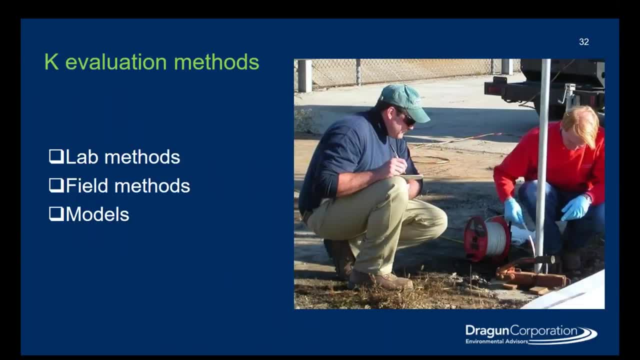 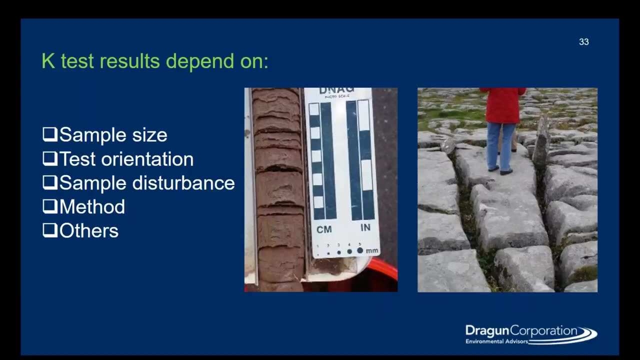 So we measure hydraulic conductivity K. There are field methods, There are lab methods, There are models And so on, And they all have their merits and demerits. But it's important to recognize that when you see hydraulic conductivity test results. 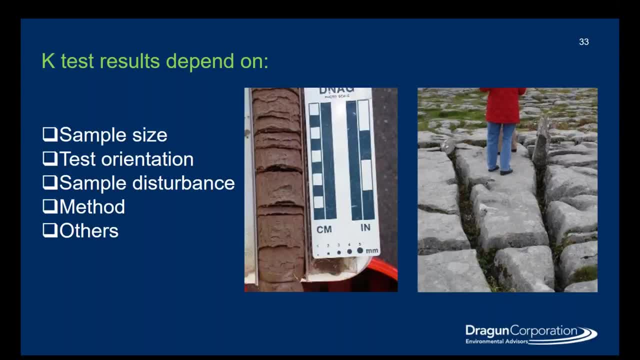 you need to evaluate how the testing was done, because hydraulic conductivity can vary with sample size. For example, if I were to measure right where my cursor is, I would have to measure. that would be a huge hydraulic conductivity. Water would move a lot. but if I moved over a little bit, 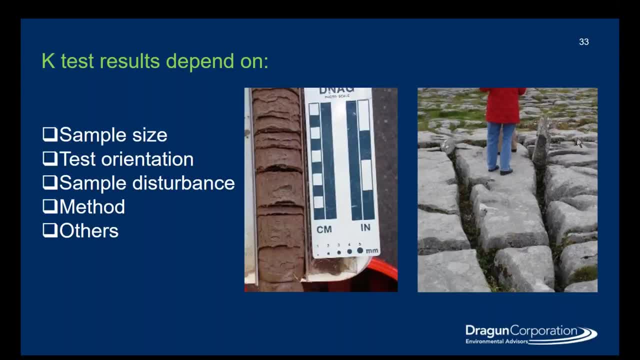 it wouldn't move much through this rock. But if I had a big sample and I incorporated that, that would give me a value that's different from just the rock or just the void space. Test orientation is important. A lot of lab tests test the amendments. 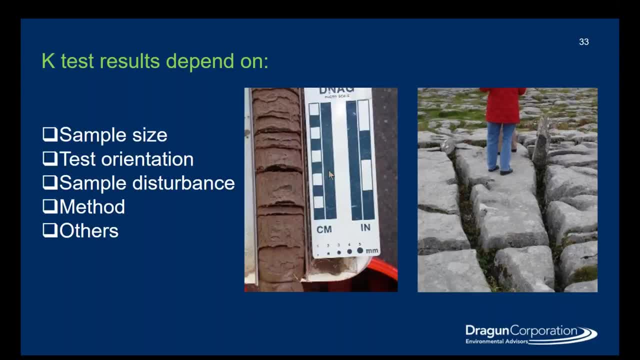 the flow vertically. But you can see in this bar of clay that the groundwater would flow readily through these permeable zones but not so readily through the clay. So lateral flow would be a lot greater than vertical flow. Some methods: you're taking samples. 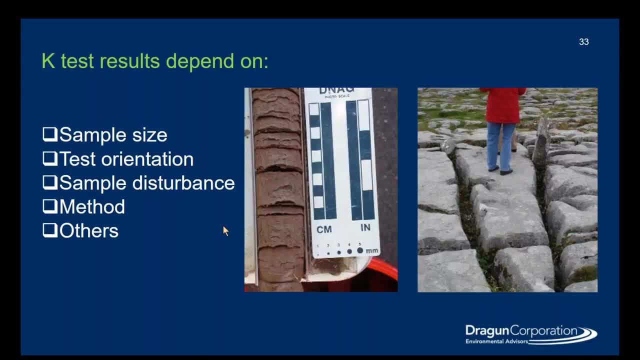 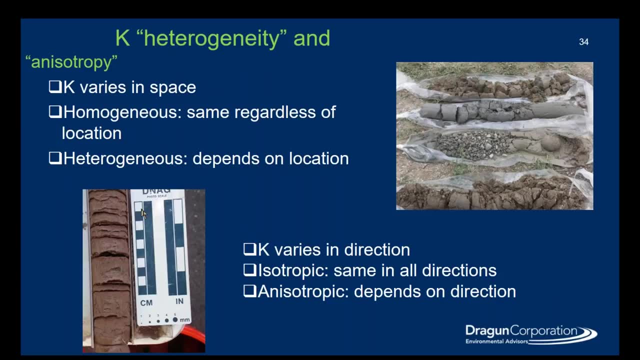 that are disturbed and they don't reflect this kind of structure. So there are all sorts of reasons why you need to look at how hydraulic conductivity testing was done. Hydraulic conductivity has heterogeneity and anisotropy, And the anisotropy talks about down here. we can see: 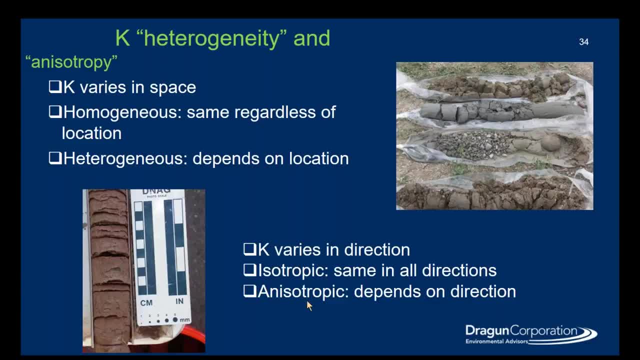 that it talks about …. … changes in hydraulic conductivity with direction And heterogeneity. talks about changes with location. So if we look at this sample, the yellow arrow is a clay soil which will have a low hydraulic conductivity. The white is a gravel which will have high hydraulic 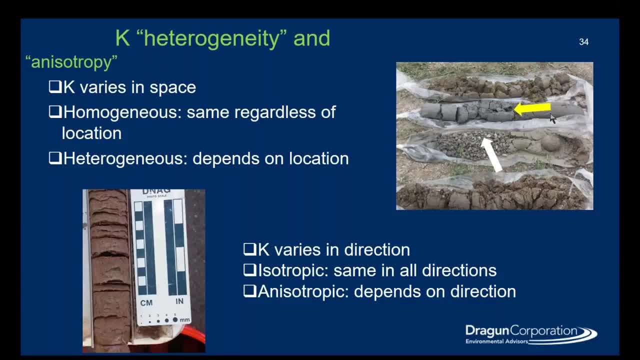 conductivity, It will transmit water. So these two areas are different. So the hydraulic conductivity varies with location. so that means that it's heterogeneous. And then the one on the bottom, the photo on the bottom. we are seeing where, if we measured vertically versus horizontally, we'd have different hydraulicemosι ductility. 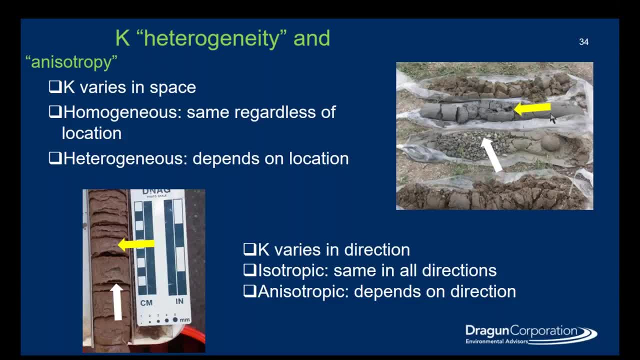 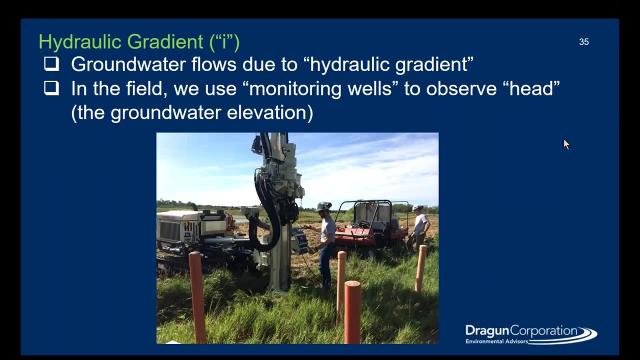 that would be anisotropy, vibrate, etc. Sorry… Anisotropy, isotropic soil, because the hydraulic conductivity depends on the direction you're measuring. Hydraulic gradient in Darcy's law is the driving force for the groundwater flow and it refers 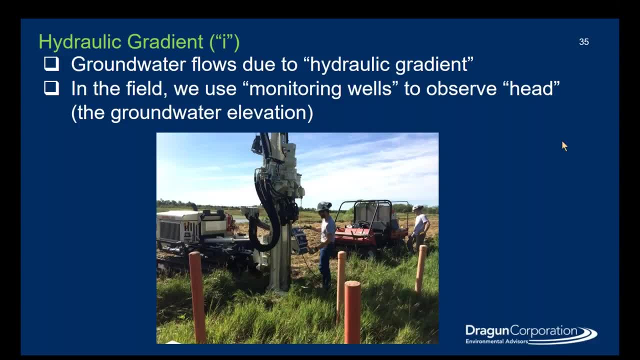 basically to the slope of the water table or some other unit that you're looking at. In the field we use monitoring wells and we can see monitoring wells in these two arrows. These other things are posts to protect the monitoring wells and in the field we measure. 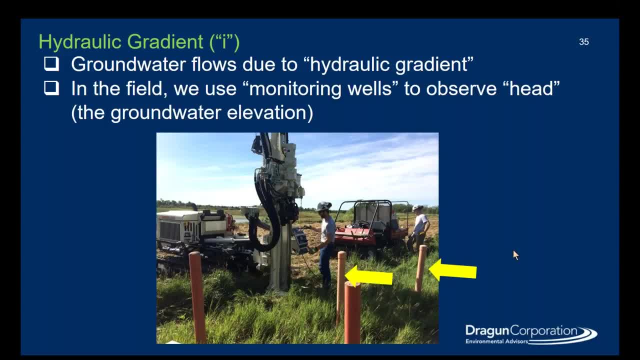 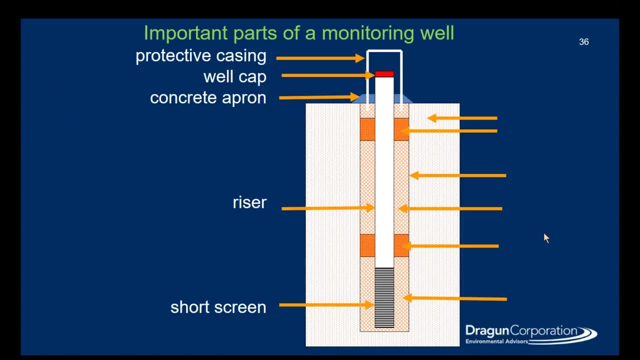 the water level and we call that the head and that's how we determine hydraulic gradient. So parts of a monitoring well that you don't see in the subsurface, there's all sorts of pieces related To the well itself. there's a screen which it allows water to move in but keeps soil out. 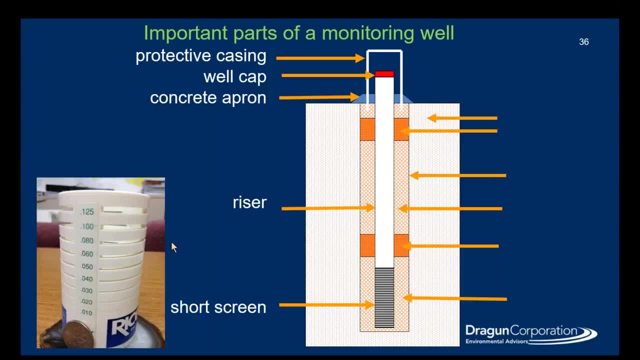 This is a demonstration screen, so it's got different size openings. The riser is just a plastic pipe or other type of material that allows you access to the screen, to the surface, and then we have some protective casings on top, and then we also have other. 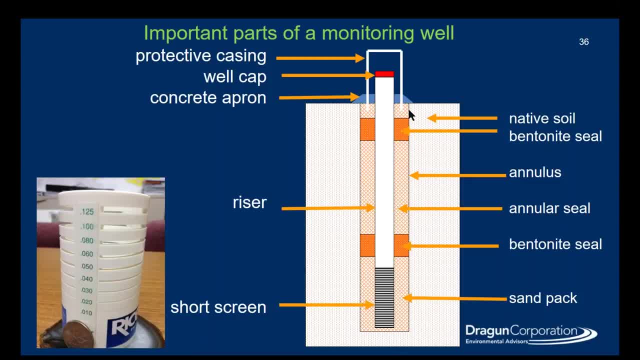 features in the annulus, which we call that space in the borehole that we put the well into, that we fill up things like a sand pack seals to prevent surface water from entering so that the screen will just sample groundwater. So if you were to measure water level, you would just open this up and see where the water level 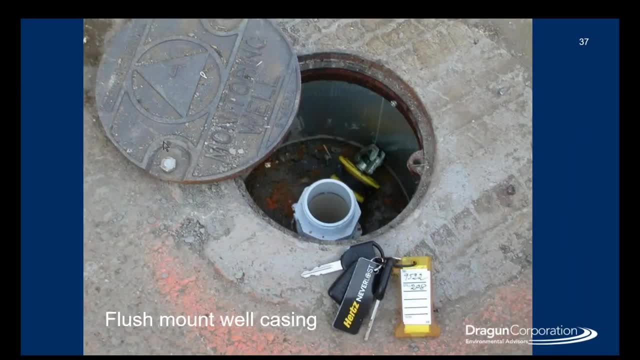 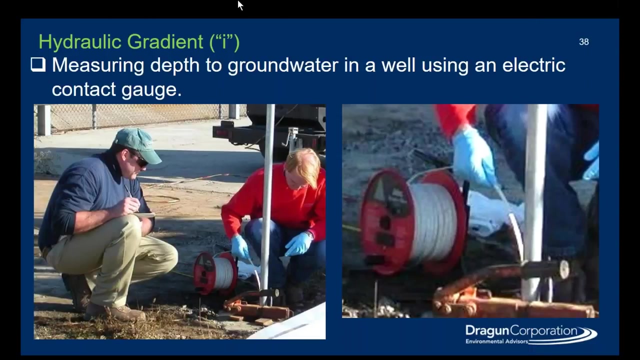 is in the well. A lot of wells that are in the field are in parking lots, so we can't have pieces sticking up, so we have these things called flush-mounted wells, and you'll often see these in parking lots around gas stations and so on, where the well is below a metal cover, And this is how we measure the water level, so we get. 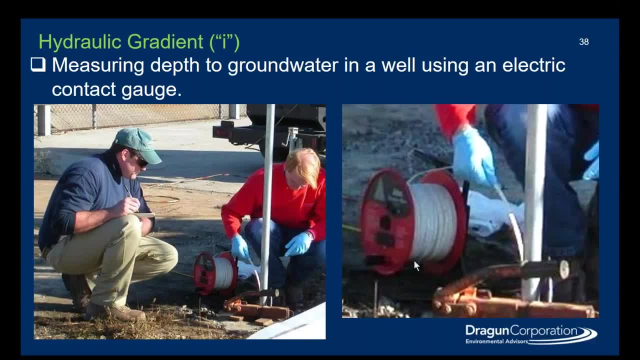 hydraulic gradient. We use what's called an electric contact gauge and that is basically got a probe on it and it's also a filter and that's how we measure the water level. So we can measure measuring tape and you determine how far down you have to go before the probe hits water When it. 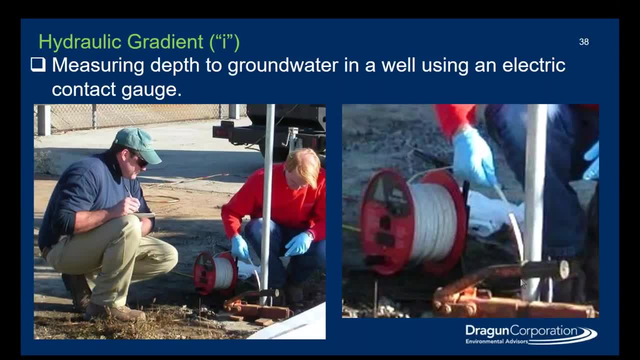 hits water, you get a buzz or you get a deflection or a electrical signal. light will go on and you can figure out the depth of water, and if you survey the top of the well you'll know what the elevation of the water level is. So we do that in a number of wells and then we plot those on a map. 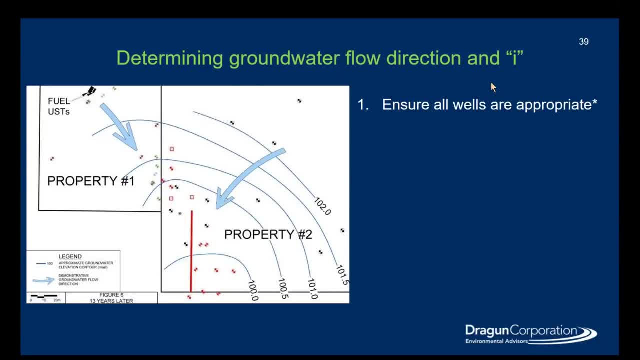 so this is how we determine groundwater flow, direction and hydraulic gradient, So we ensure that all the wells are appropriate. In this example, all these symbols are wells, and what I mean by appropriate is that the wells are in the same, are of the same depth and in the same. 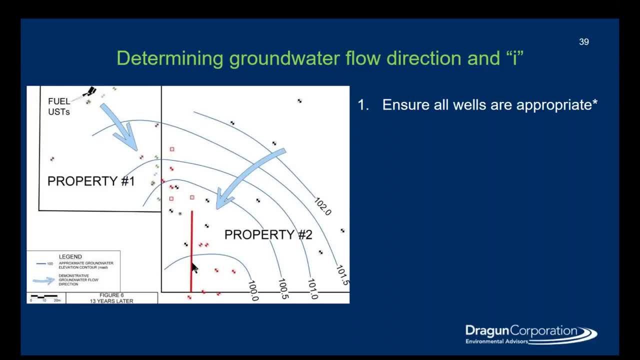 formation and often people make mistakes. or sometimes people make mistakes and include wells that are in different formations and different depths. So we plot the groundwater elevations on the map and contour the data, join points of equal elevation and these are the contours here: 102,, 101.5 and so on. 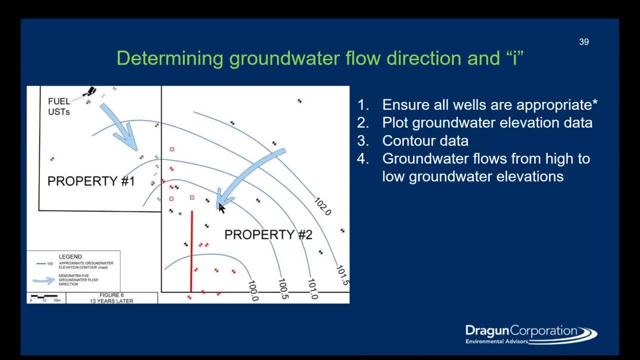 and then groundwater flows from the high elevations to the low elevations in terms of the groundwater contours, and the contours are drawn perpendicular. so when we look at this line it's not really a great example, but these lines should be perpendicular: the arrow and the contours. this one's a little better up here. 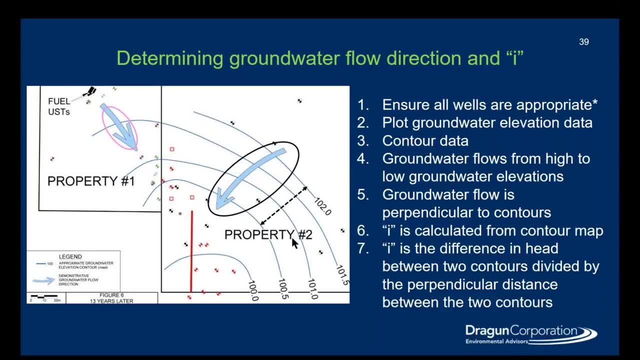 And then I is calculated from the contour map and basically we take the difference between the values of two contours and divide that by the distance between these locations perpendicular to the contours, and that would give you your hydraulic gradient they can use and Darcy's law. so we have 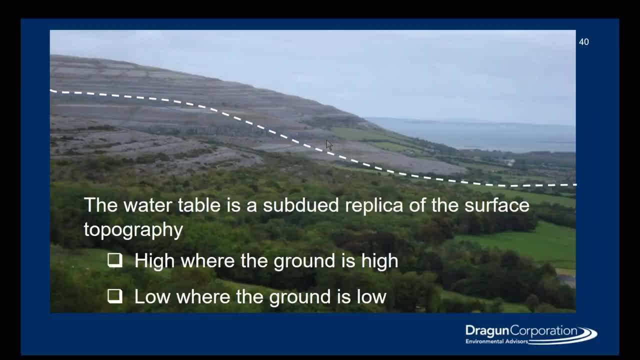 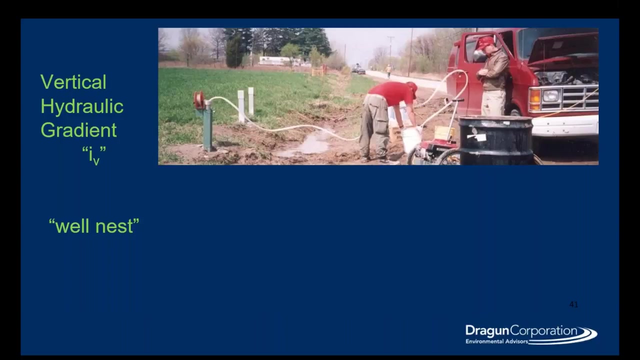 groundwater flow direction and hydraulic gradient. so the water table is a subdued replica of the surface topography. that means where the weather groundwater, where the topography is I, the ground water is high and the where it's low, the groundwater is low, so we can use a vertical. 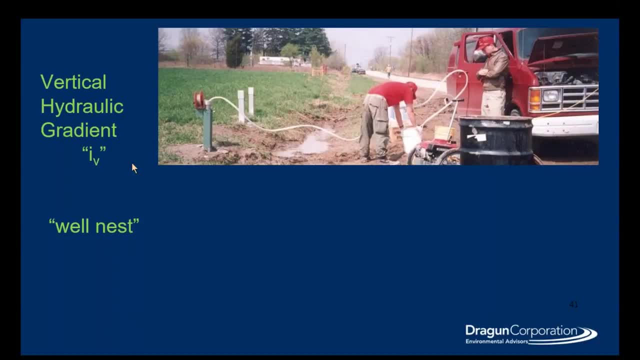 determinant vertical hydraulic gradient, also using a series of wells where the well screens are at a different depths. so here we've got a one well with the screen at that depth, another one at that depth, and we call this a well nest. so if in the well nest the deeper well has the lower, 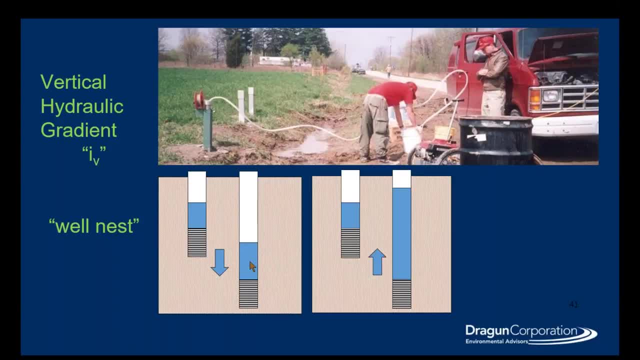 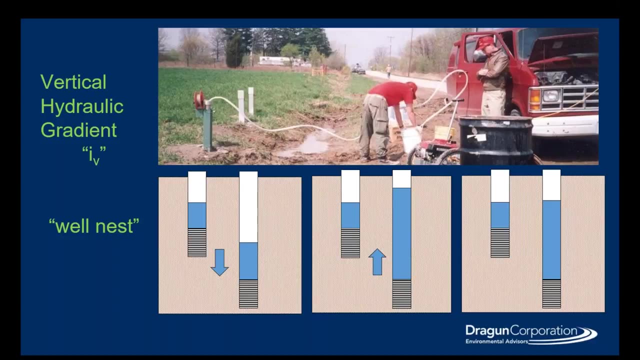 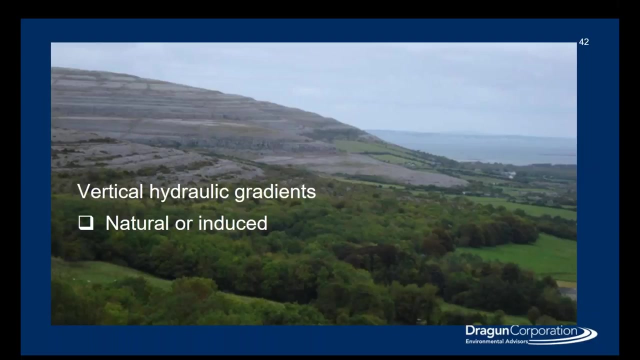 water level, that's considered a downward vertical hydraulic gradient. where you've got a situation where the deep well has the highest water level, that's called a an upward a vertical hydraulic gradient. if you don't see a difference, that means there's not a vertical hydraulic gradient. so if we go back to our topographic picture, we can have vertical hydraulic gradients. 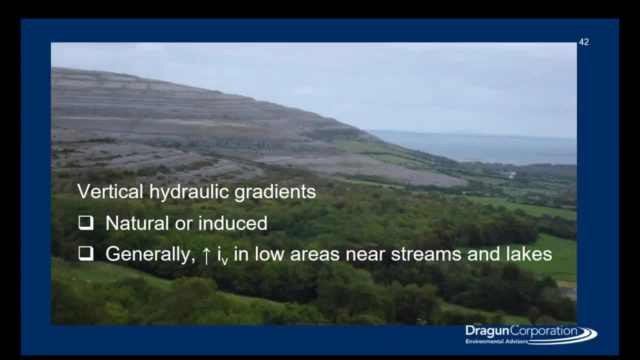 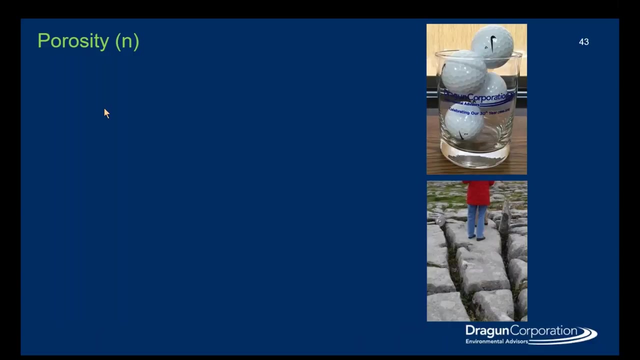 that are natural or induced. and in terms of natural condition, generally we find that in low areas the hydraulic gradient is upward, so generally near streams and lakes, and in high areas, like hilltops and so on, you generally have a downward vertical hydraulic gradient. so just looking at porosity and in jarcey's law, pores are openings in soil or rock. 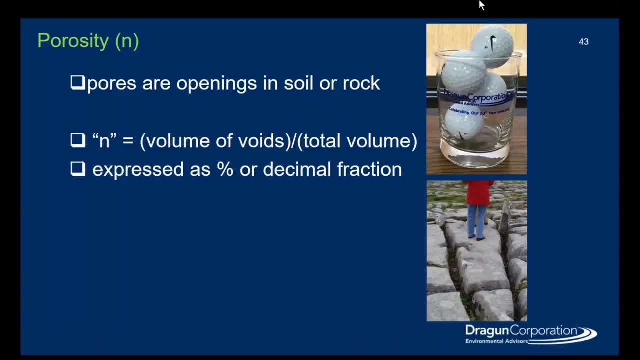 porosity- n is a symbol we use- are the volume of voids of the total volume. so if we looked at this glass, that would be the total volume and the void space would be between the golf balls. uh, porosity is expressed as a percent or decimal fraction. it could be primary or secondary porosity. primary means it's. 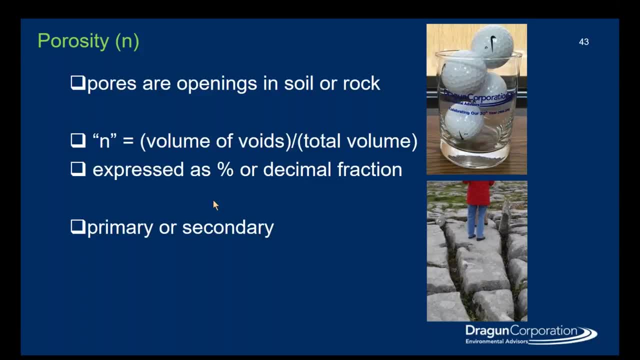 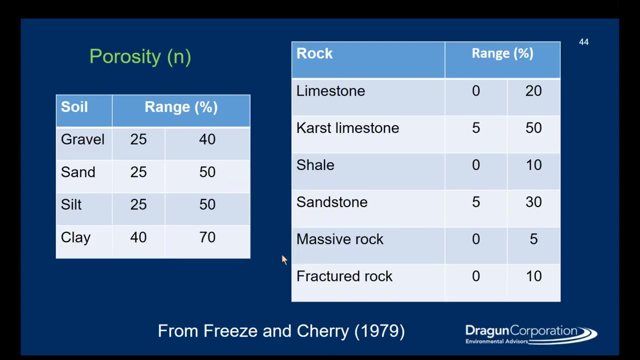 created when the rock or soil is created. secondary means it's created afterwards, like we see in this bottom slide where the rock is fractured. we commonly use tables to assign porosity. rarely do we see people actually measure porosity and practical groundwater problems. so these are some tables. 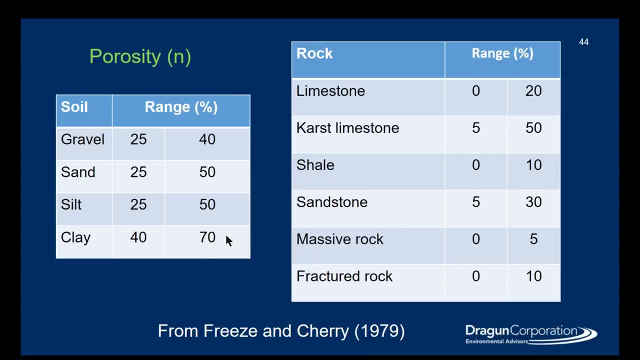 from the textbook by freezing cherry porosity with ranges for different grain sizes of soil and different types of rock. and you see, fractured rock is potentially has a lot of uh of porosity, and massive rock doesn't karst limestone, just means it's like caves. um, but the thing to notice is porosity. the variation is much smaller than what we saw hydraulic conductivity like interconnected porosity is what we're interested in. um, but another thing to notice is porosity. the variation is much smaller than what we saw hydraulic conductivity, and then that's what we're interested in. what we're interested in and the other question: in terms of the gravity that we're looking at, so maybe it's a little bit different- of the overnight resting dolomite rock- we're most likely to use high Members of the science about this, but rather than what we saw- hydraulic conduct in the area of the body, land and other types of rock. 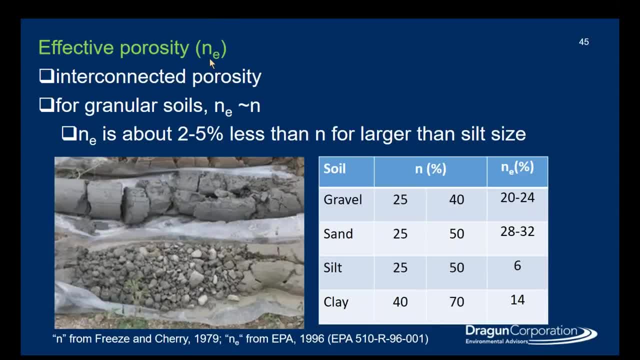 well, there are a few areas of rock that has some of that in some places like we're interested in interested. That's the symbol, And for granular soils, like the gravel that we see in here, there's not much difference between the total porosity and interconnected porosity. There is a 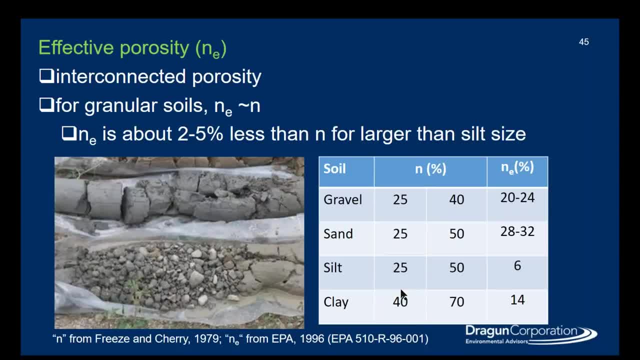 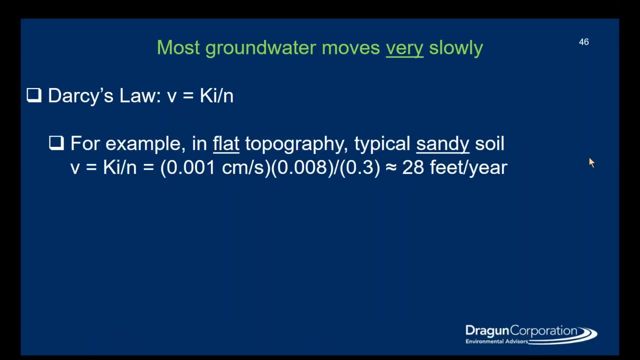 large difference for clay soils, as you can see in this table comparing porosities and effective porosities. So most groundwater moves very slowly. Darcy's Law of Velocity is equal to hydraulic conductivity times hydraulic gradient divided by porosity. And I've just worked on two examples with kind of typical values. So typical hydraulic. 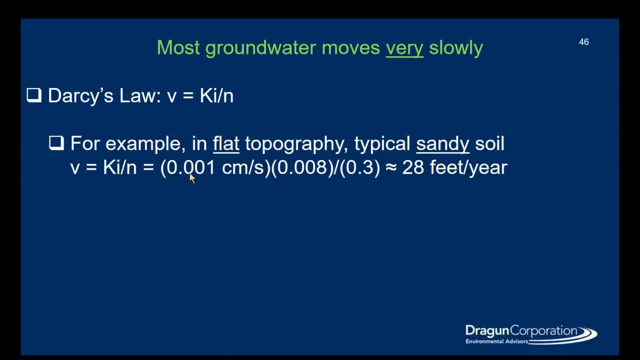 conductivity for a sandy soil would be 0.001 centimeters per centimeter of soil. second hydraulic gradient in a flat topography might be 0.008 and a porosity might be 0.3. that would give us a a velocity of 28 feet per year. that's. 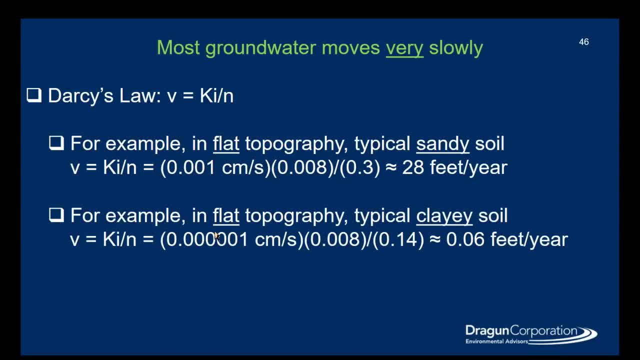 the velocity of the groundwater. for a clay soil, where the hydraulic conductivity is much lower, you can see we've used the typical clay soil: effective porosity. the groundwater moves point zero, six feet per year. that's very small amount. so geology which affects the hydraulic conductivity, will affect. 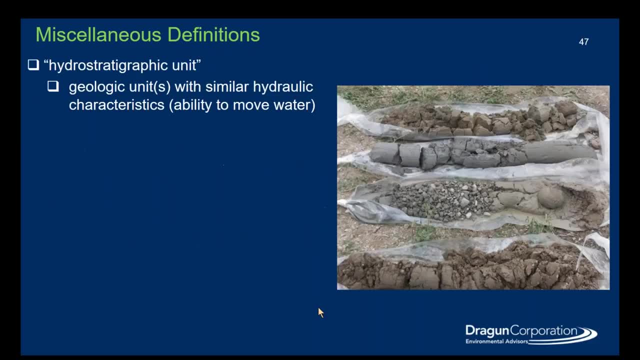 how quickly groundwater will move in the subsurface. so some miscellaneous definitions. one of the things that we often talk about, our hydrostratigraphic units. these are geologic units or layers with similar hydraulic characteristics or similar abilities to move water. so an aquifer would be something like the. 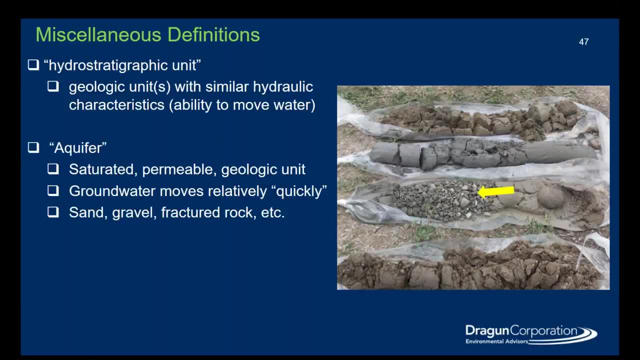 gravel we talked about it's saturated, permeable geologic unit where the groundwater moves relatively quickly, for groundwater and things that are aquifers are like sand or gravels or fractured rock or some types of sedimentary rock might be aquifers. an aquitard is a saturated, permeable geologic unit through which groundwater moves slowly. 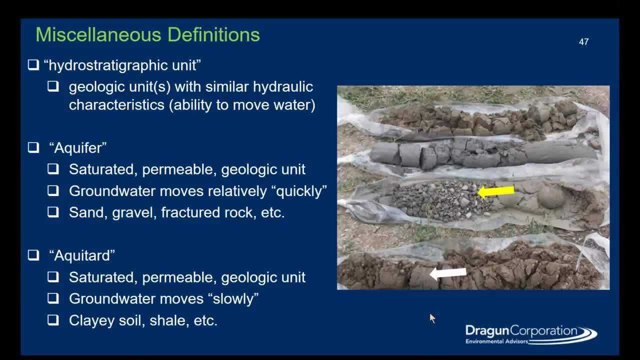 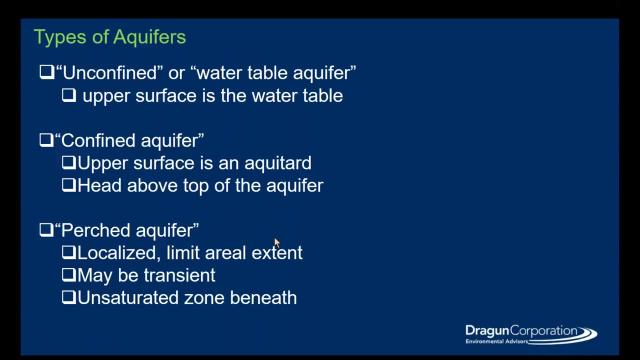 things like clay soils, like we see in the white arrow shale, which is the type of rock that is clay also- would be an aquitard, so commonly act for aquitard. there's other types of hydrostratigraphic units, but these are the two most important ones, and aquifers can be different varieties and this: 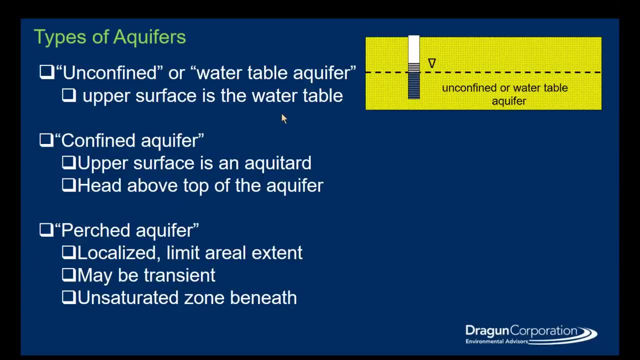 will affect the likelihood that an aquifer might be contaminated. for example, an unconfined or impunded water table is one where the uh upper surface of the aquifer is open to the atmosphere, so this would be like sandy soil all the way to the surface. 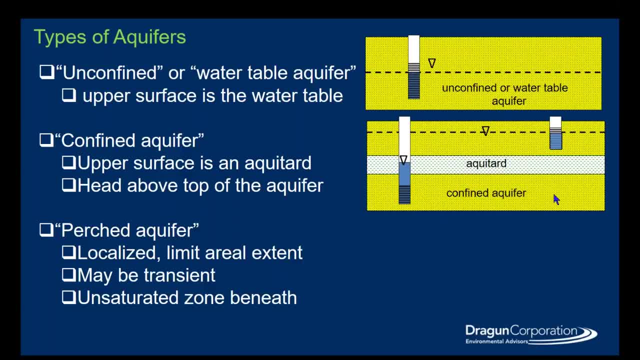 there'd be no clay soil above it. for example, a confined aquifer is one where the aquifer is overlaimed by an aquitard, basically protected by the aquitard, and the water surface is not so much dieses. the vegetation has to be käytauf. 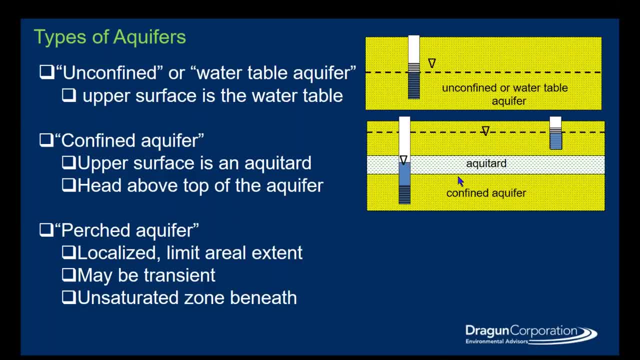 but for any kind ofки is determined by the state, stayed there and no water table would. eveninteitk is considered a height in the case of cloud, at this point it would userection や levels usually above the top of the confined aquifer, and these are very. 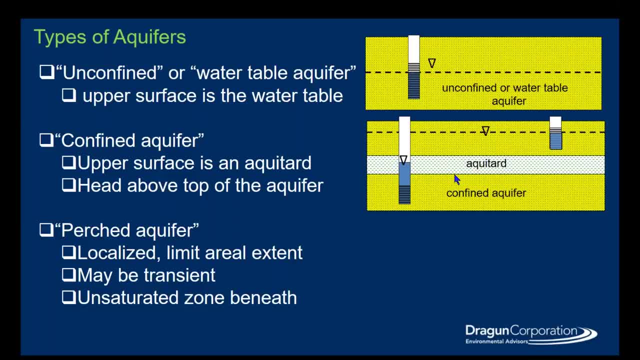 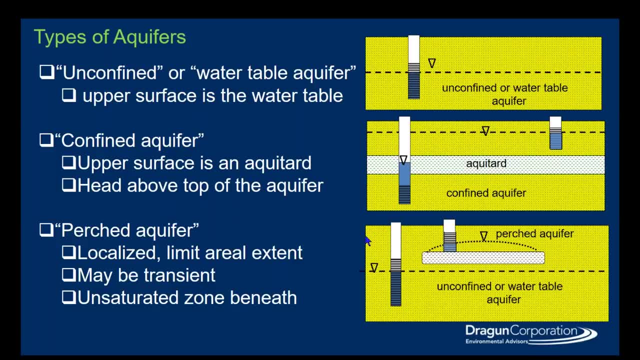 important distinctions when it comes to things like pumping water out of a well, how these behave to behave quite differently. and a perched aquifer is a situation where you might have a low permeability layer above the water table that would cause a perching of a saturated soil. This may be transient and you would find 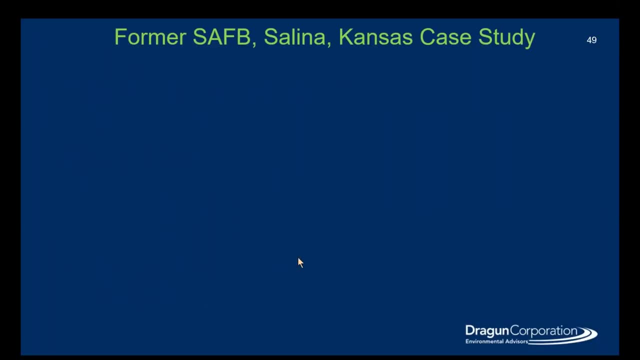 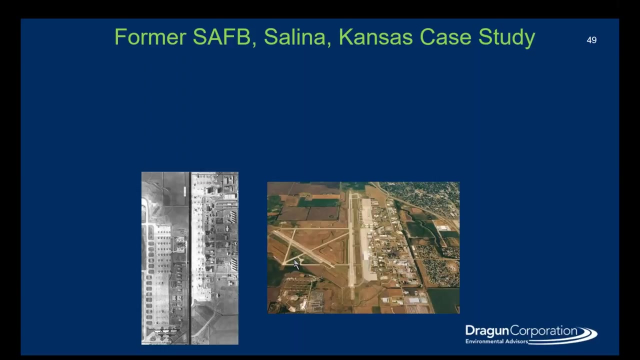 unsaturated soil. So getting back to our example which we talked about at the beginning, the former Schilling Air Force Base in Salina, Kansas. you know it was an active military base in the 40s, 50s, 60s and it's now a an industrial center and 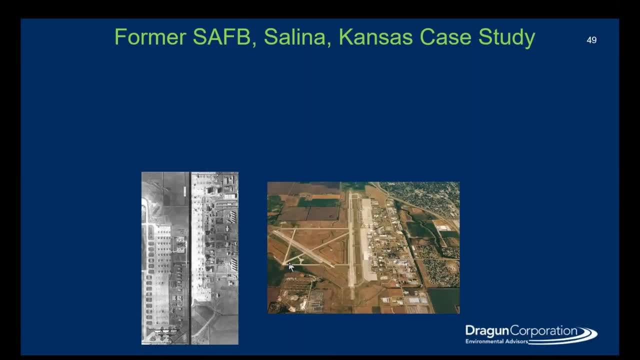 an airport and people live there. People live around it, People work around it, and what we wanted to know was: where are the chemicals now? In the 1960s they were using hundreds of drums of TCE per month. Where did that go? What directions of the chemicals are moving We, we know. 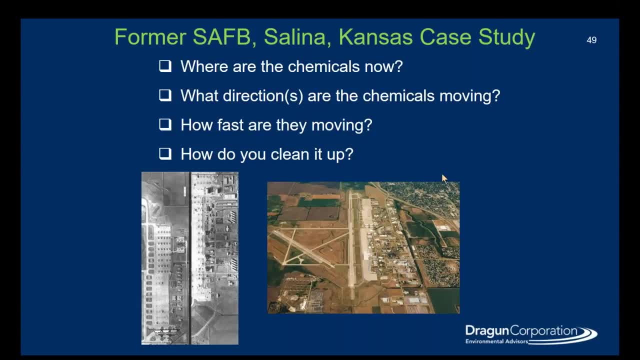 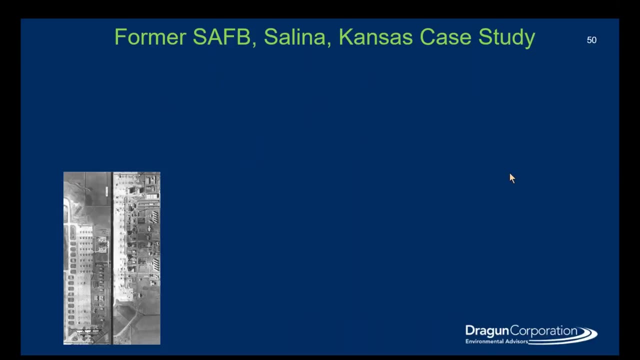 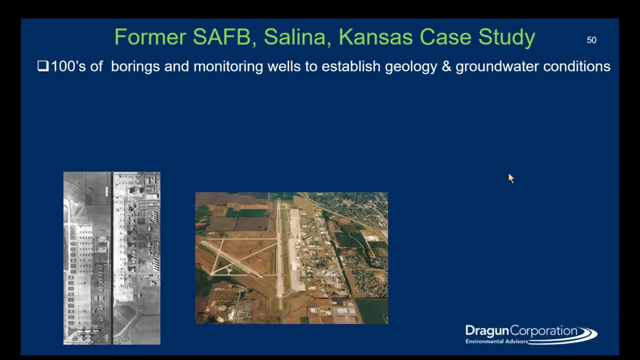 that the the city wells are to the northeast of this location. How fast are the chemicals moving and how do you clean it up? So in order to do that, we looked at the site and we put in hundreds of borings and monitoring wells to establish the geology and the groundwater conditions. See where the 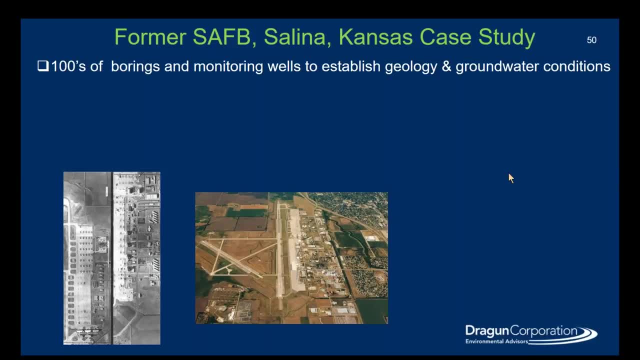 permeable zones are, where the one zones that aren't permeable are, and which direction, where the groundwater flowing, how fast those are flowing. We were also, with this data, able to put our arms around both the sources. We knew what, where the sources were and the plumes of groundwater impacted groundwater that. 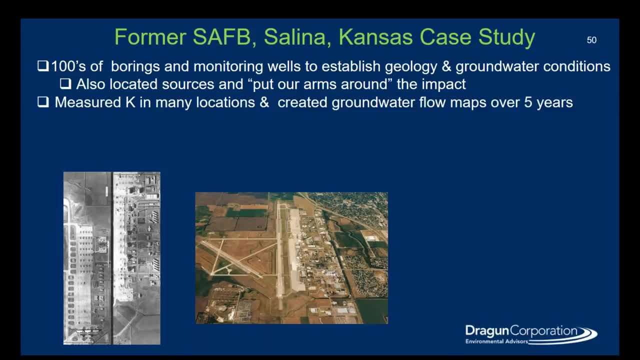 left the sources. We measured hydraulic conductivity in many locations and we created groundwater flow maps over a period of five years, So how fast the groundwater is moving and we know in what direction it's moving, because we've got all the groundwater heads measured and mapped out. So the next step was to develop a conceptual 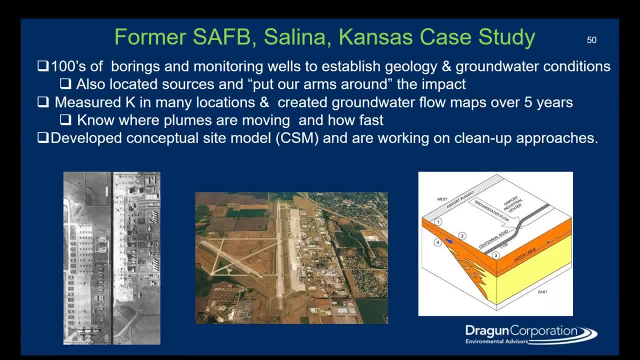 site model, which we talked about in one of our earlier sessions and that looks something like this: on lower right hand corner, where we generalize the geology so that we can come up with methods that will be effective and cost effective in cleaning up the contamination that started in the 40s and